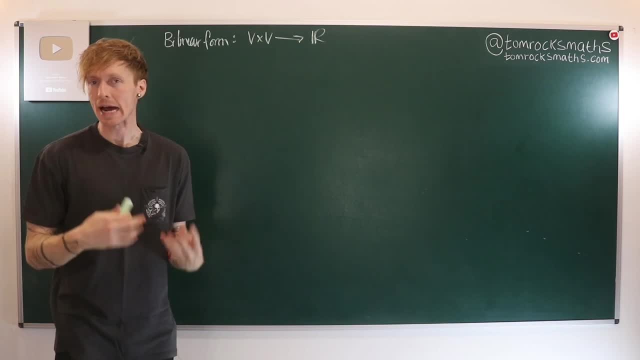 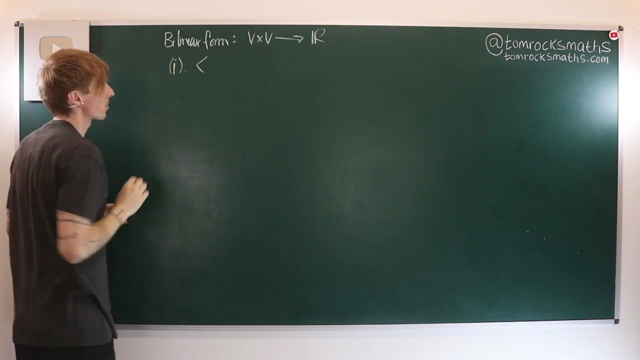 properties in order to be defined as a bilinear form. The first property we want in our map is that it must be linear in the first variable. So written out formally, that's going to say that if I take the inner product which is going to 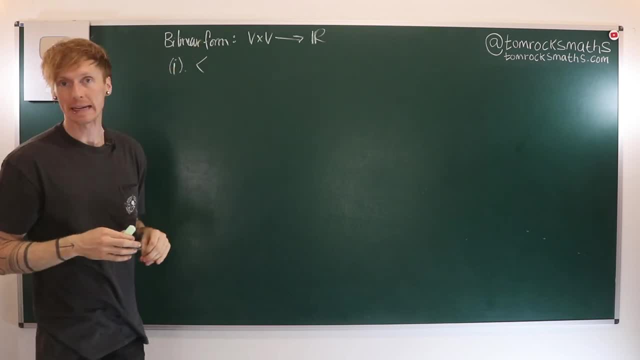 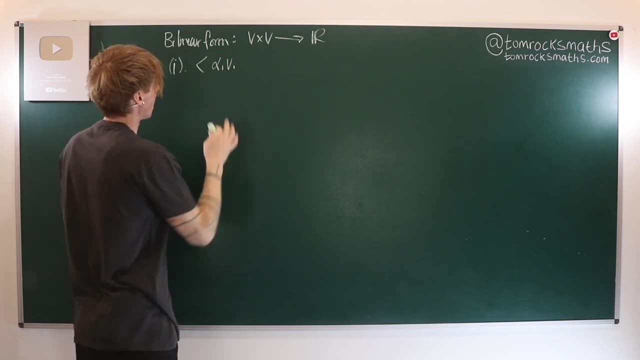 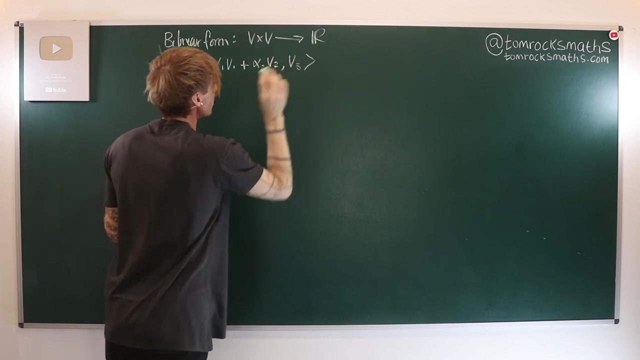 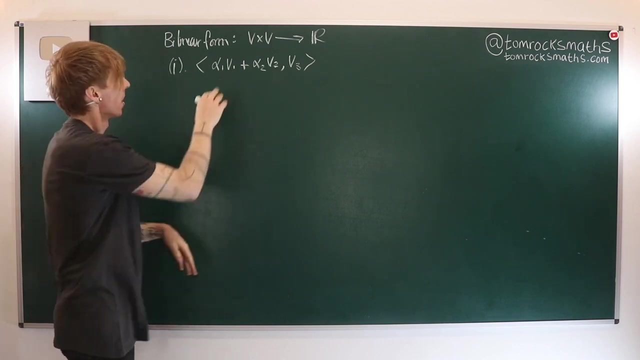 be defined or written using this angled bracket. So if I take a linear combination in the first position, so let's suppose it's some scalar alpha1, V1, plus another scalar alpha2, V2, and we take the inner product of that with V3. So just to note here: V3 is a vector in the space V. 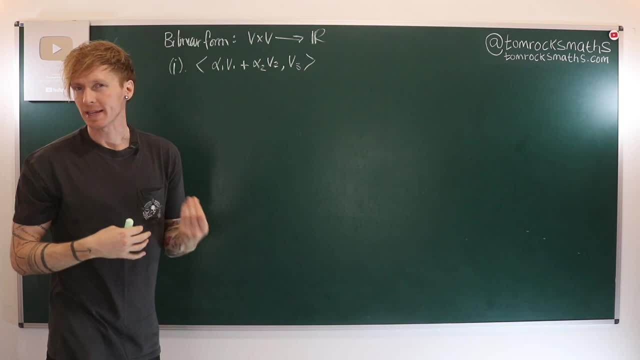 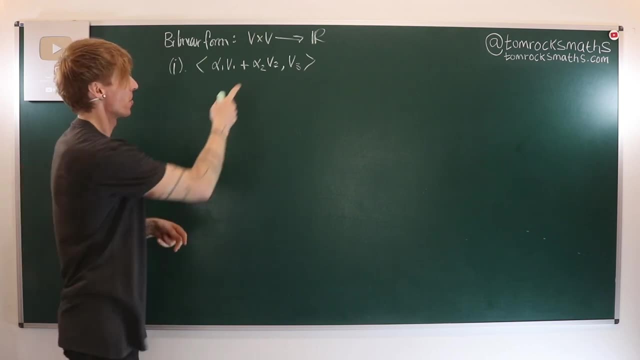 V1 and V2 are also vectors in the vector space V and since we know vector spaces are closed under addition and subtraction, scalar multiplication, when we take this linear combination of V1 and V2, we know that also belongs to V. This is all implicit at this point, as these are: 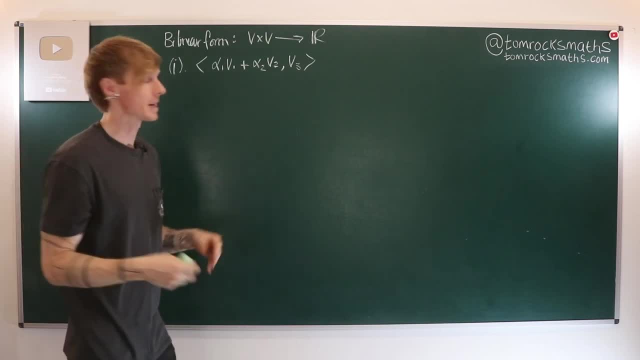 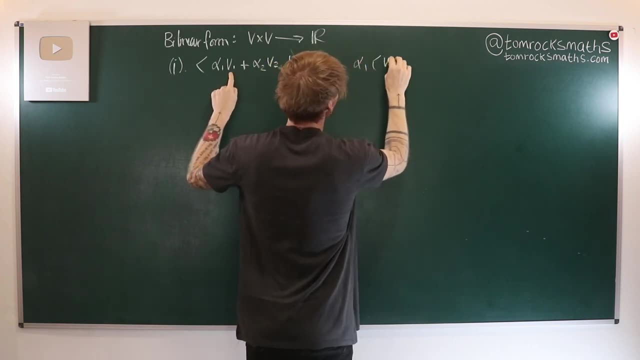 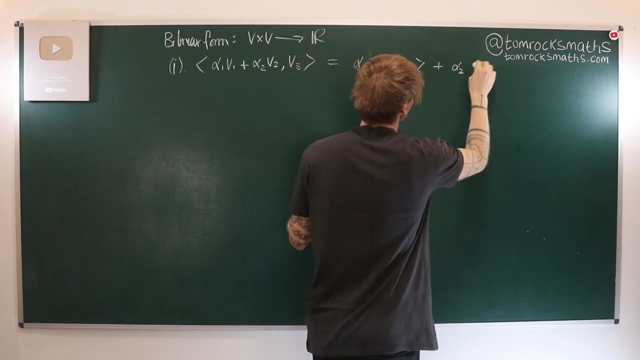 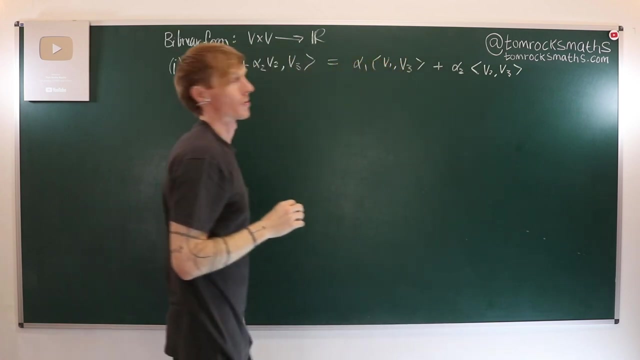 things we've hopefully established by now. So we need this to be equal to, for linearity, alpha1 times the first component, V1 comma V3, plus alpha2 times the second component, v2, again in a product with v3.. So this is going to be: 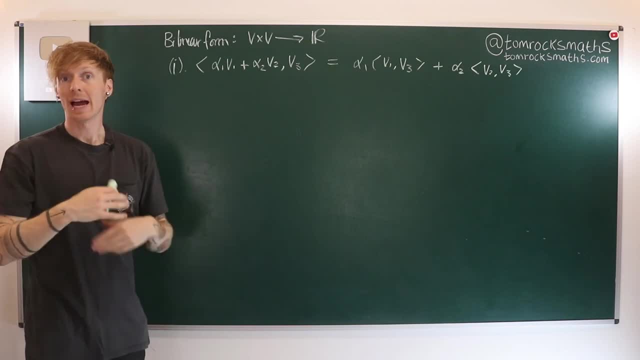 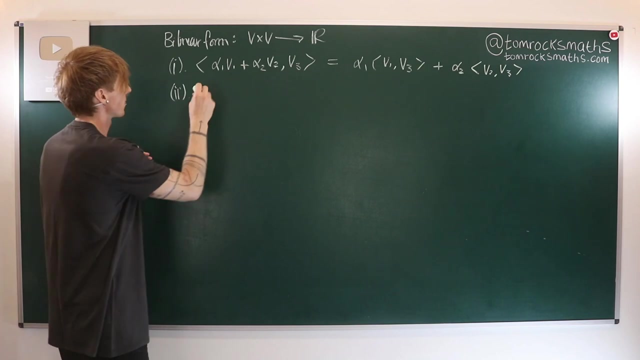 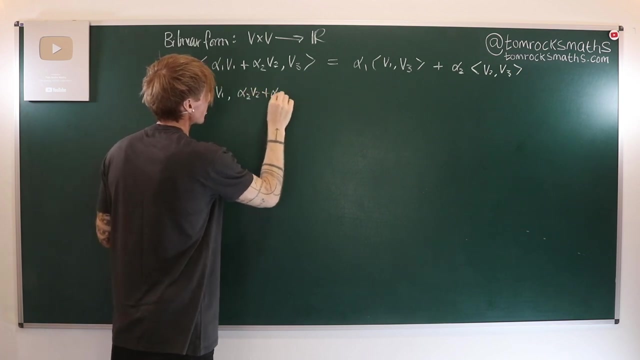 linearity in the first position and then the second property that we must have for the bilinear form is going to be as follows: Very similar, but now we want linearity in the second position. So here we might have something like v1 comma, alpha 2, v2 plus alpha 3, v3 in a product is the same as if we were to pull out. 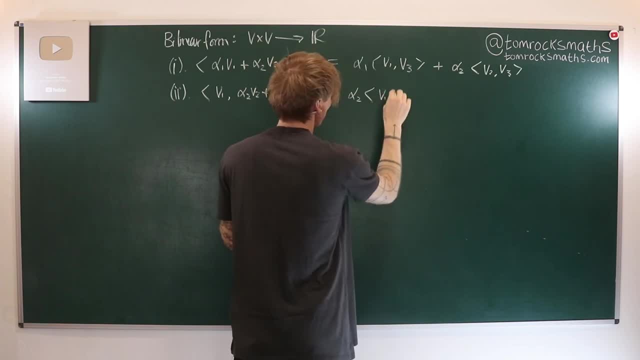 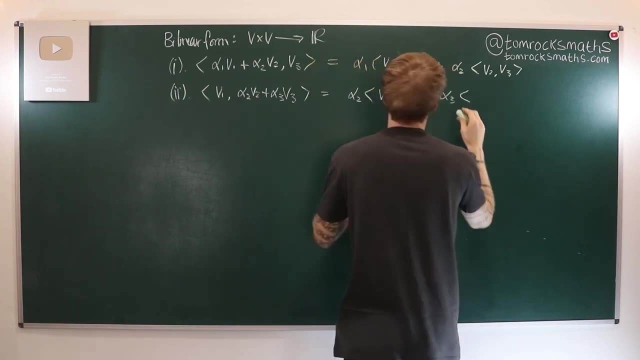 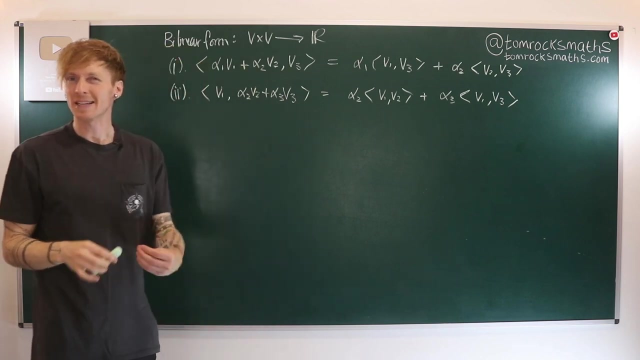 the alpha 2 and take the inner product there with v1 and v2, and if we were to add that to alpha, 3 times the inner product there of v1, v3.. So they look very similar but it is important that we realize the. 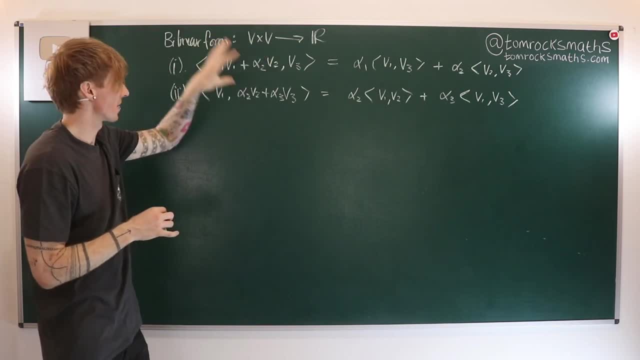 first one is already linear and so it's only going to be linear. So we now have to find the integral of that first integral of v1 and v3.. So now we just have to. one is linearity in this first position and the second one is linearity in the second position. 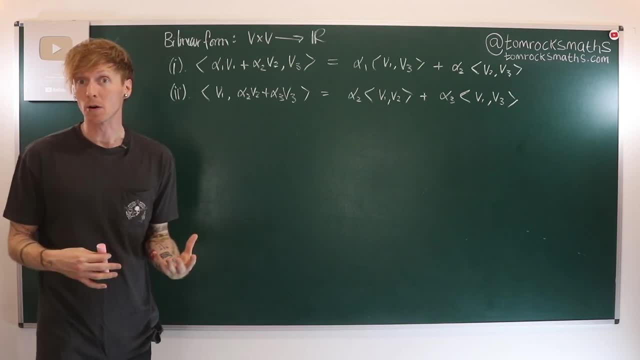 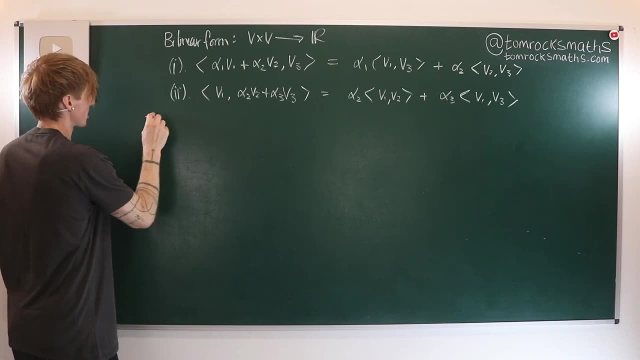 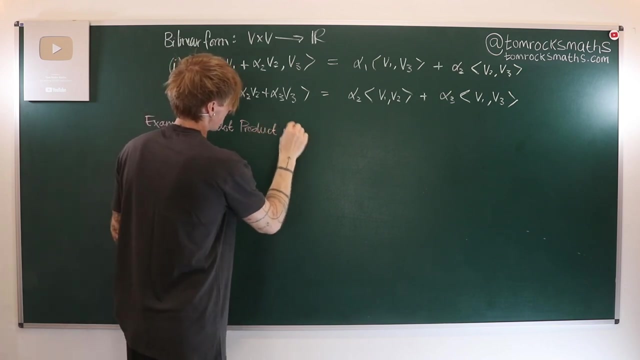 Perhaps the most common example of a bilinear form is actually the dot product, which I imagine most of you are already familiar with. So let's call this example one the dot product, and we'll take this in our n, our standard n-dimensional wheel vector space. So here, if we 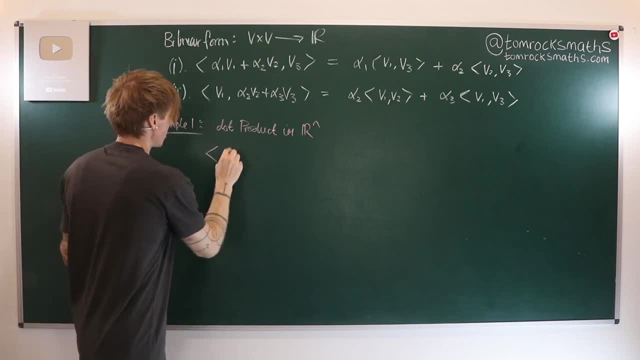 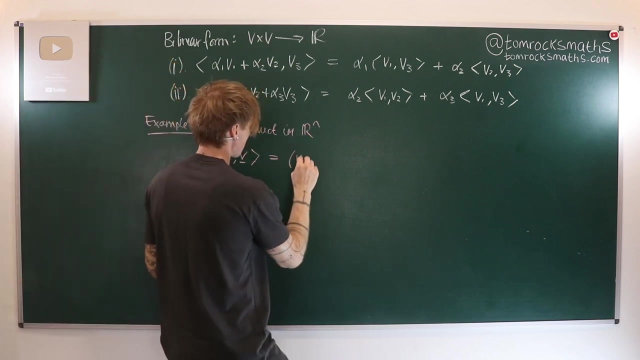 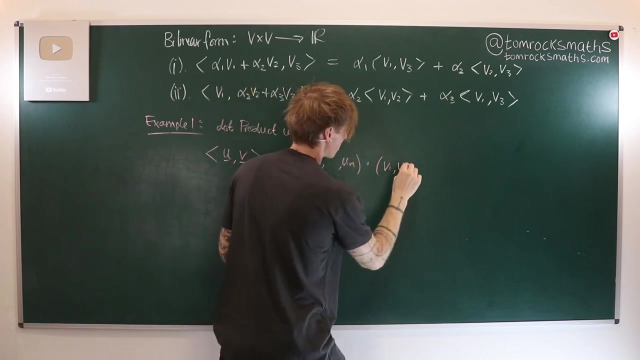 have two vectors. let's suppose we had u and v and we were to take that inner product, then we would simply define this exactly as we would define the dot product. So we could say: well, this is just the same as u1, u2, dot, dot, dot up to the nth entry. dotted with v1, v2, dot, dot, dot up to the nth entry. 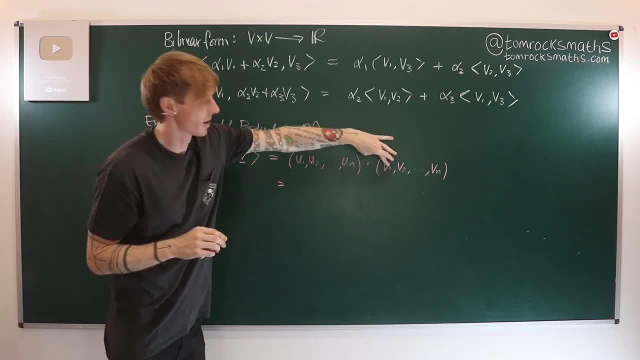 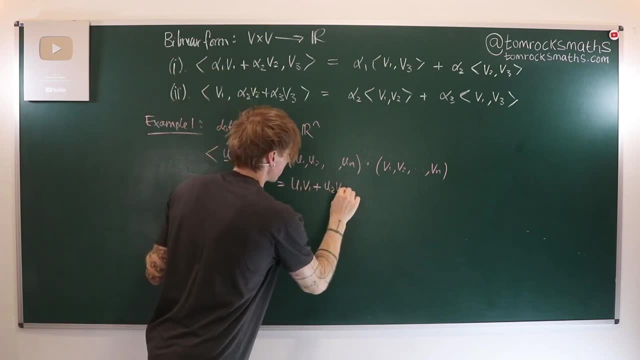 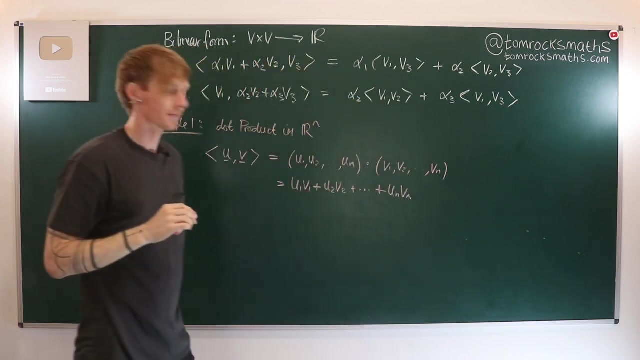 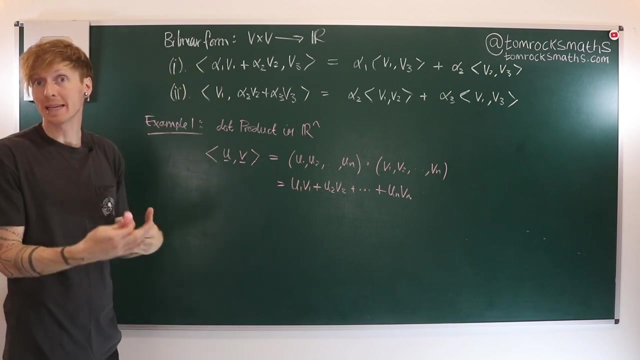 and of course the dot product means we multiply together component-wise and then add them. So this would be u1 v1 plus u2 v2 plus dot dot dot plus u n v? n. Now we want to check that this does indeed satisfy our two properties in order to be. 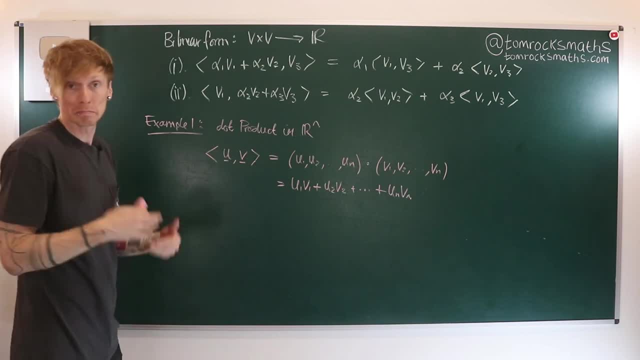 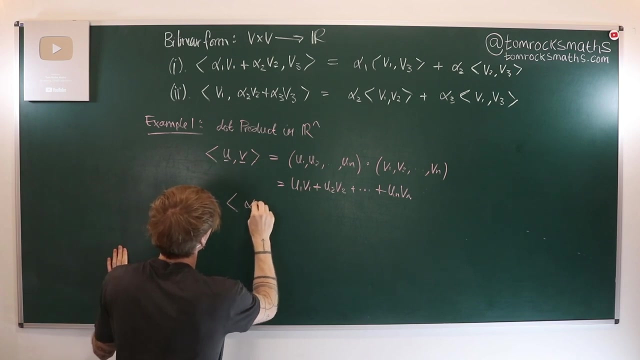 declared a bilinear form. So let's consider an example. So we'll just look at the first position for now, but the second one will follow in the same way. So if we were to consider, suppose we have now alpha1 u plus alpha2 v. 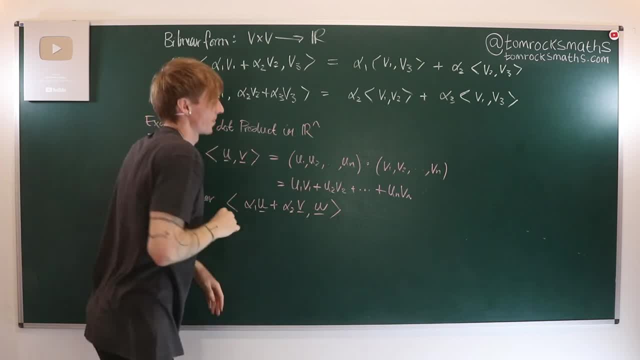 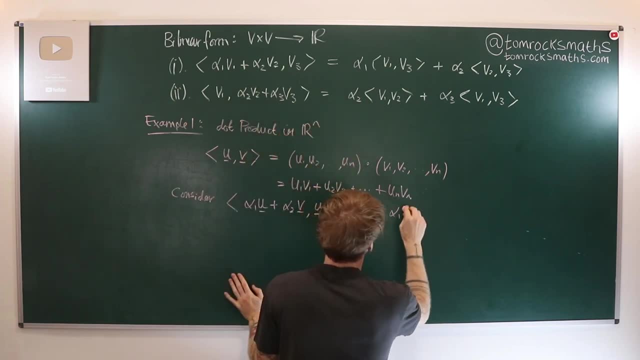 And we take that product with w, Then, using the definition of the dot product, we just say: well, that's the same as alpha1 u plus alpha2 v dotted with w. But then if we were to write out all of those component by component, the first one is going to be alpha1 u1 plus alpha2 v1, all the way up to: 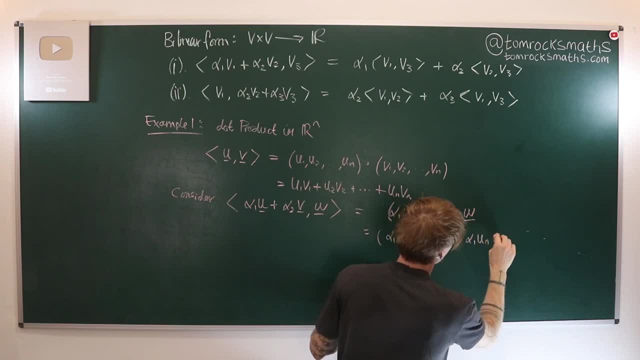 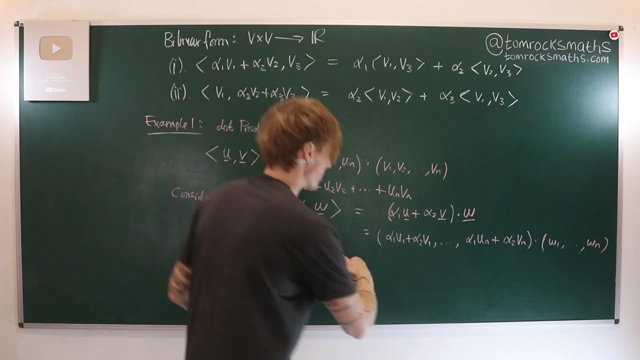 the same thing: alpha1 u- n plus alpha2 vn dotted with w, which is w1 up to w n, And now we just multiply out using the rules of the dot product. So it came to give me this whole of the first thing. So we've got alpha1 u1- w1 plus alpha2 v1- w1. 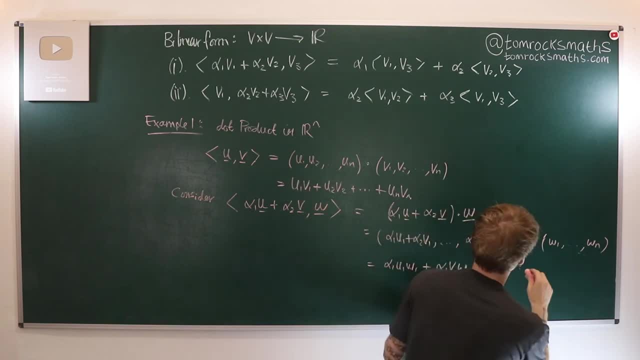 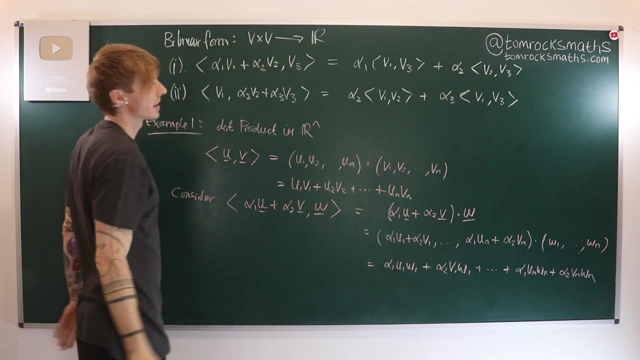 plus all of the in between terms, and then finally alpha1 u n w n plus alpha2 v n w n. Now this is the expansion of the left hand side here, of number one. So now we need to think about what would these look like, these two pieces? But fortunately we can. 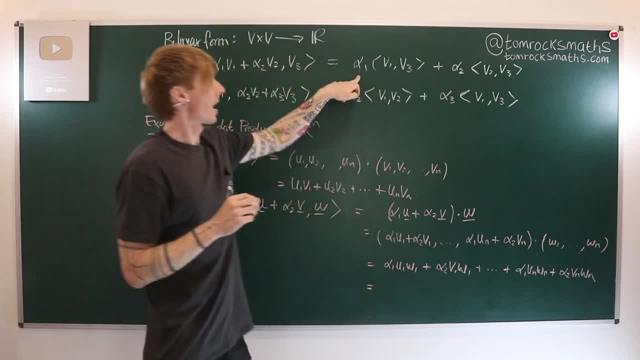 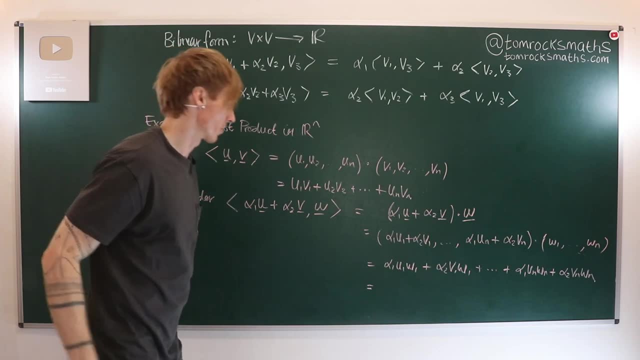 just group it together to see that. So we can see that alpha 1 is pulled out at the beginning, our scalar, and similarly we want all of the terms multiplied by alpha 2.. So if we group those together we bring out alpha. 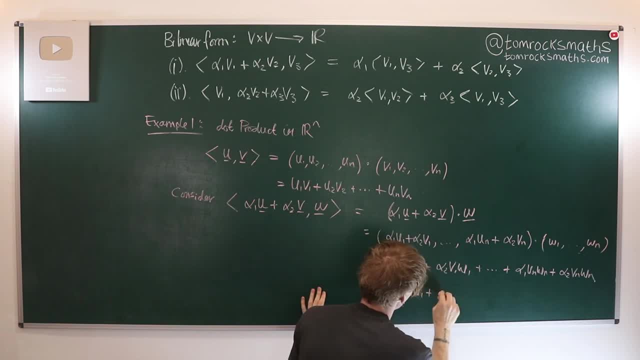 1, and then we're left with u1 w1 plus dot, dot dot up to u n w n. And similarly we get the alpha 2 comes out, and then we've got v1 w1 plus dot, dot, dot plus v n w n. 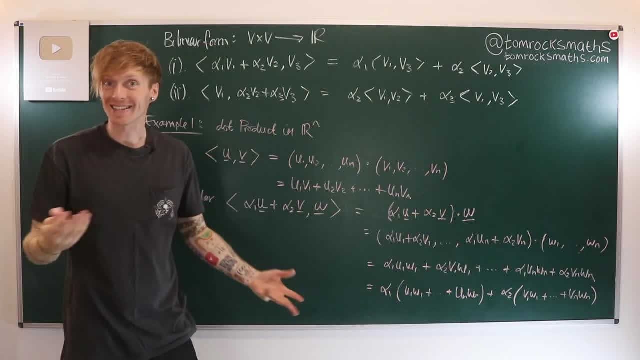 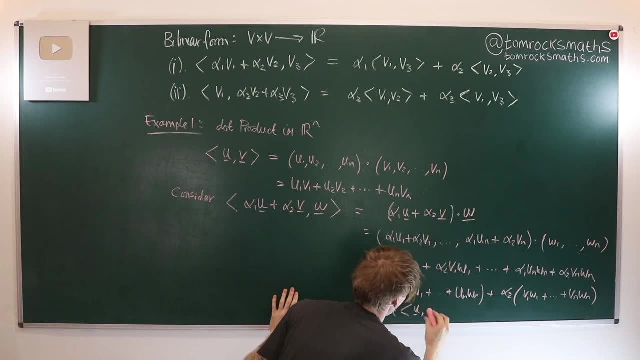 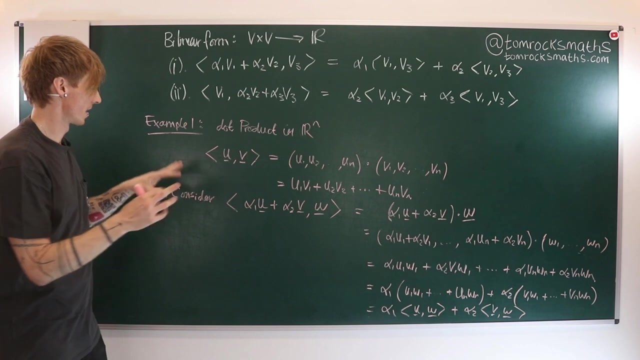 But what do we have in those brackets? It's exactly the dot product, those individual pieces. So this is alpha 1 u with w plus alpha 2 v with w, where again the inner product is defined via the dot product. So we can see that number 1 is. 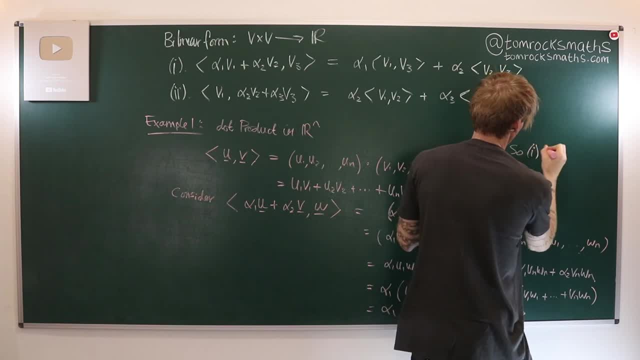 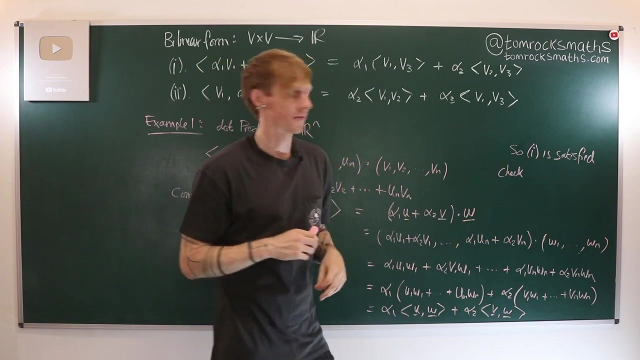 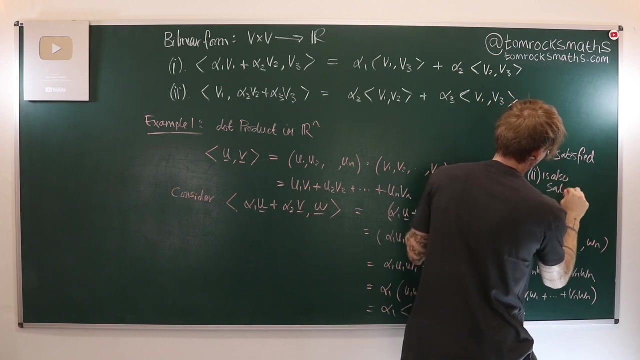 satisfied. so I can say so 1 is satisfied And you can also check- and you should do this as an exercise if you're new to bilinear forms- very good way to get to grips with the definition. So check that 2 is also satisfied. 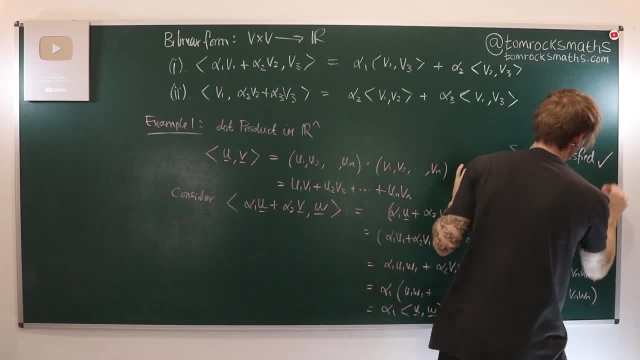 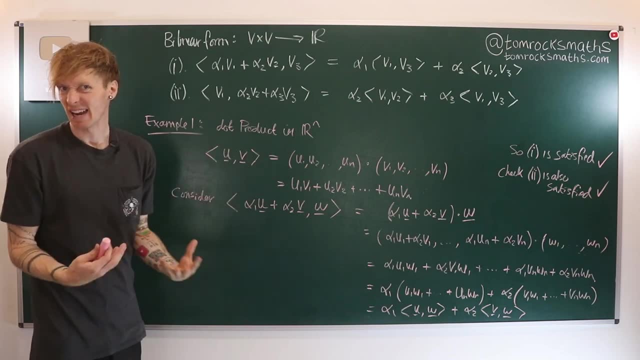 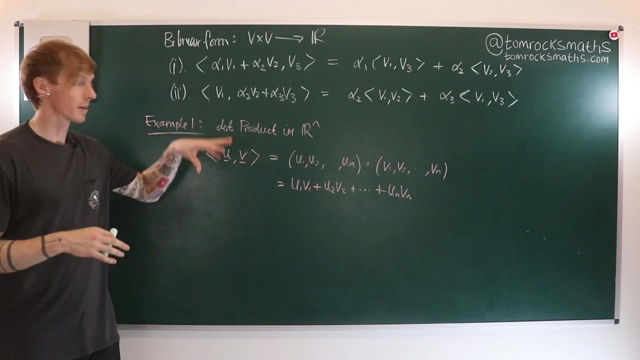 So you'll find that both of them hold. therefore, we can conclude: the dot product is indeed our first example, our most simple example, I would say, of a bilinear form. Now, you may have noticed in the previous example with the dot product that were we to swap the order, were we to swap the rolls here of u and 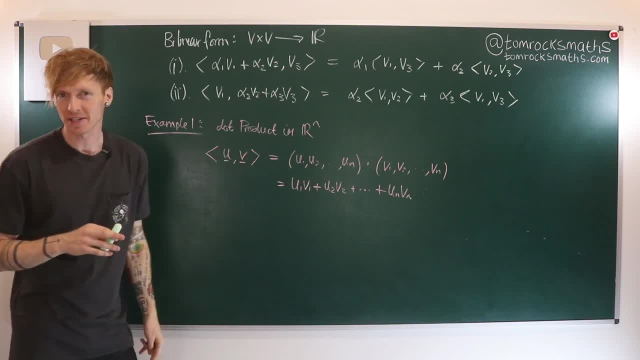 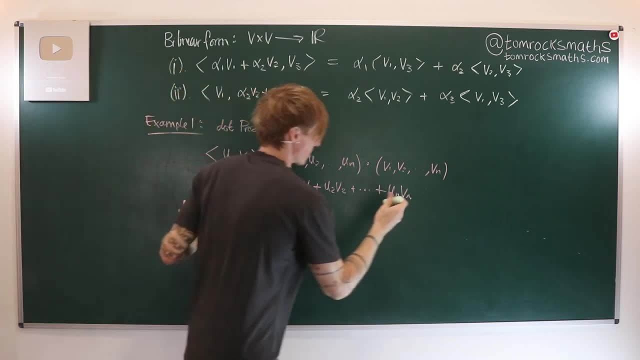 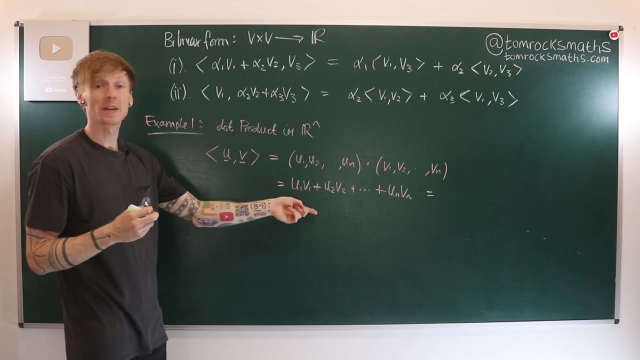 v. so to put v in the first position and u in the second position, we would in fact get the exact same product here. So we could in fact say: well, this is actually the same. because of the commutativity of the real numbers, u1- v1 is the same as v1- u1, we can multiply in any order. 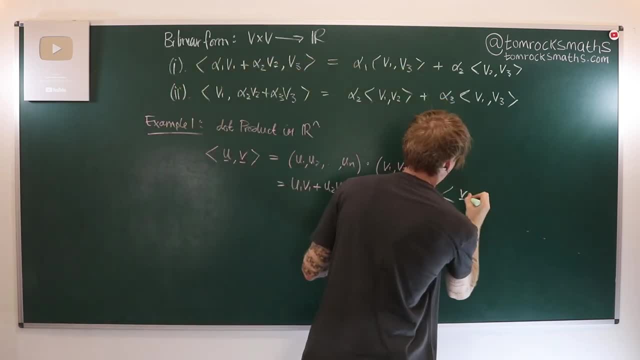 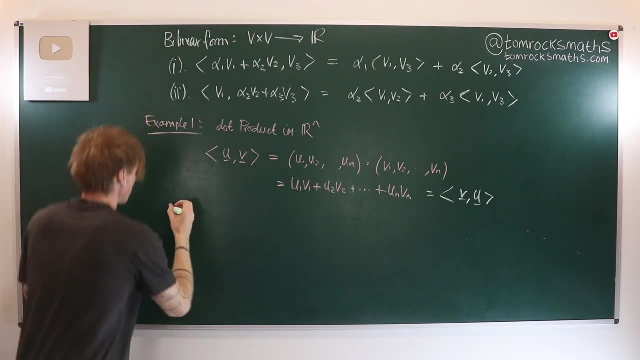 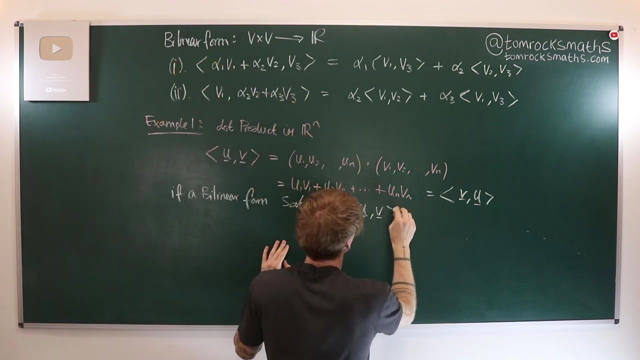 So this is actually the same as if we had v and u and, more generally, if we have a bilinear form which has this property. so we can say: if a bilinear form satisfies what we would call symmetry, so u v is equal to v and u. 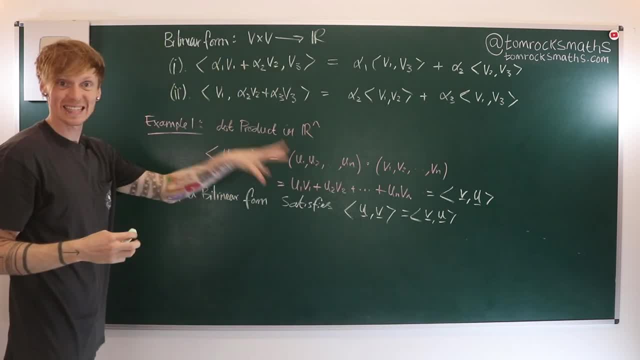 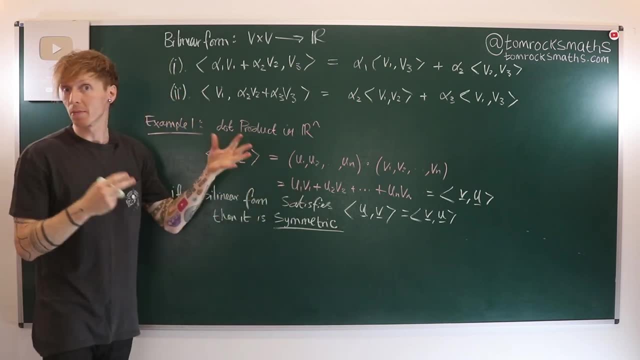 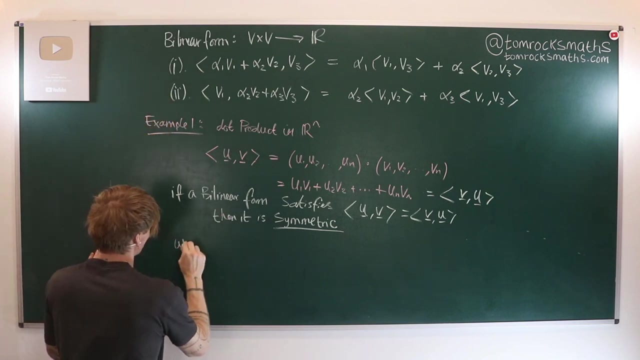 if this holds, so, if a bilinear form satisfies this, then it is symmetric, And again we can see that this is true for the dot product by explicit calculation. Now there is another important property, which is called positive definite, Which we should also think about at this point. so we say a bilinear form. 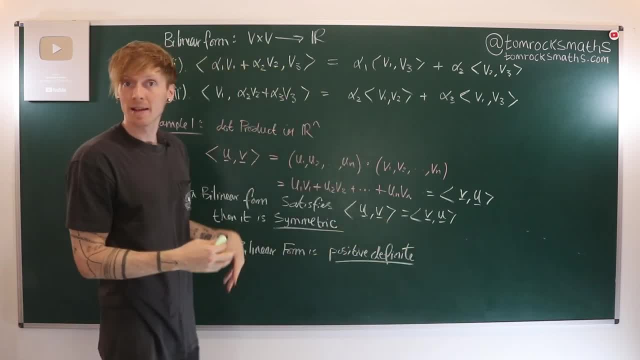 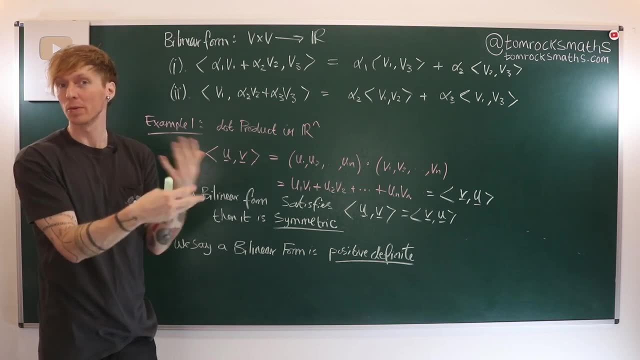 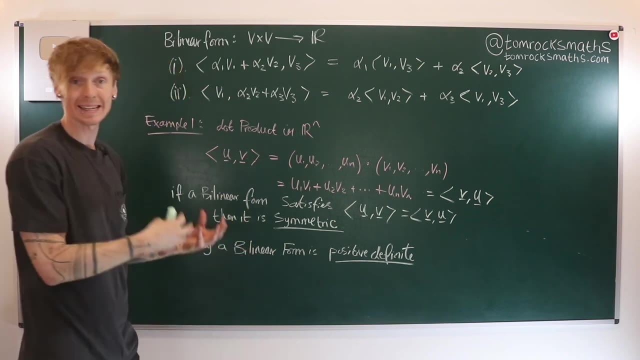 is positive definite To mean that when you take the bilinear product of the same thing, so of u with itself, then the answer is always positive or always non-negative. So explicitly writing that out, it means we say a bilinear form is positive. definite that 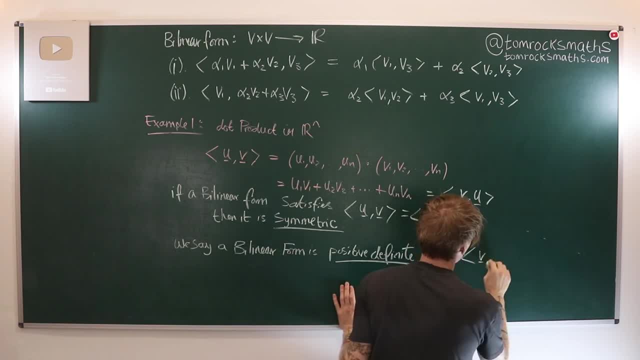 means or is equivalent to saying that the inner product or the bilinear form of V with V is greater than or equal to 0, and this is for all V in our vector space. and just to go back and be complete, I probably should have set up: 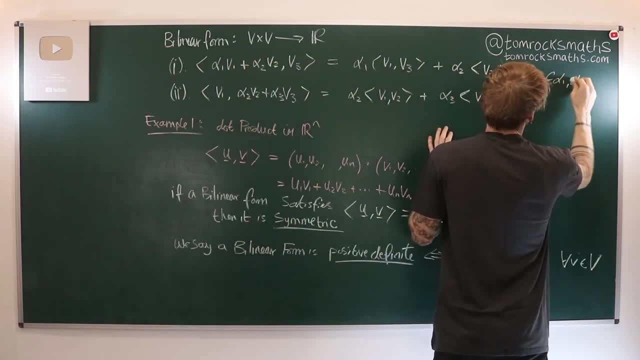 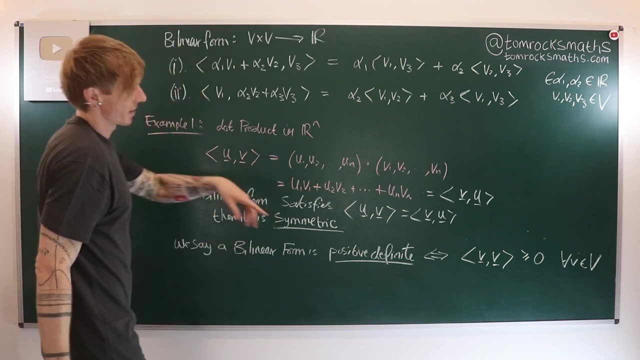 here that this is true for all alpha 1 and alpha 2 in the reals in our field and for all V1 and V2 and V3 in our vector space V. but hopefully you figure that out by this point. So we say it's positive definite if this is greater than or 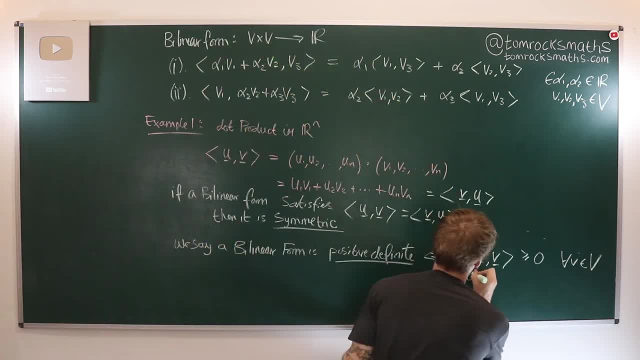 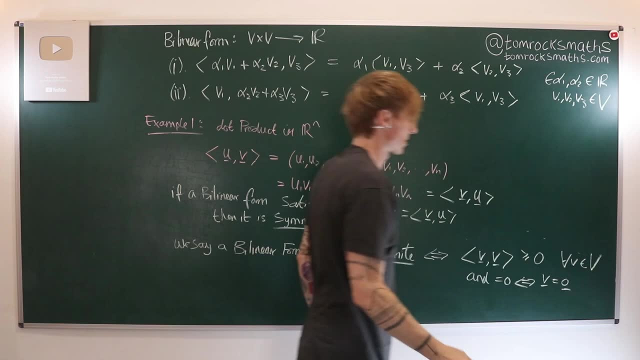 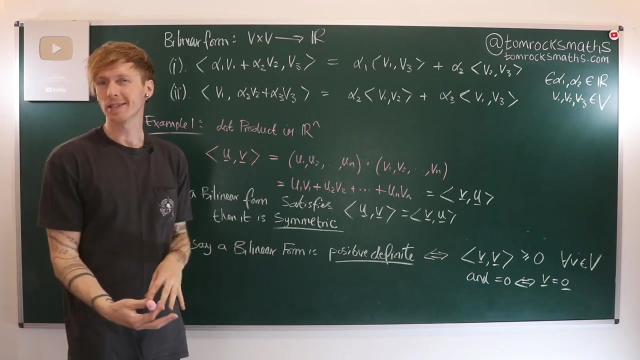 equal to 0 for all vectors V and in fact equal to 0 if, and only if, the vector itself V is the zero vector for that vector space. So if we now look at this positive, definite property in the context of the vector space V, we can see: 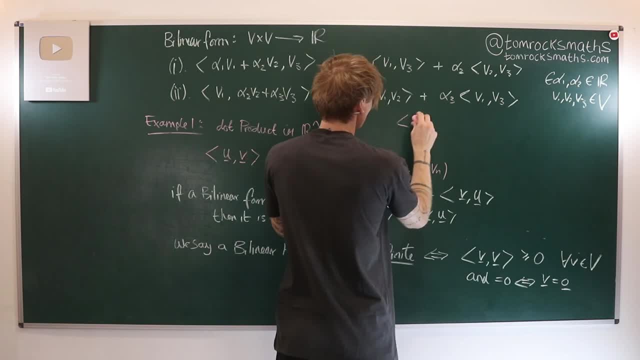 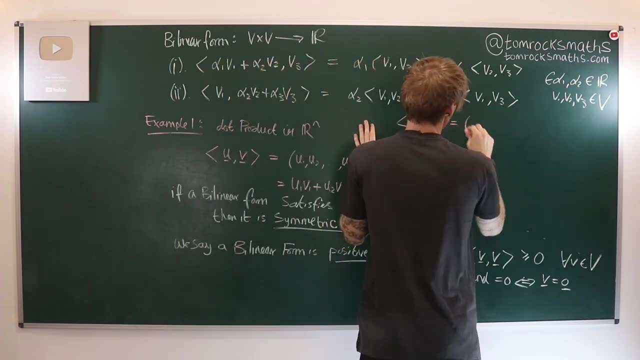 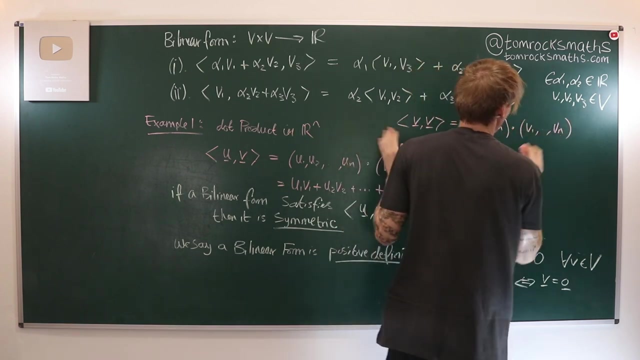 that if we look at the x-axis in the context of the dot product, then we will see over here that if we take the dot product of two vectors which are the same, so that's the dot product of V1 up to VN, dotted with V1 up to VN, then that 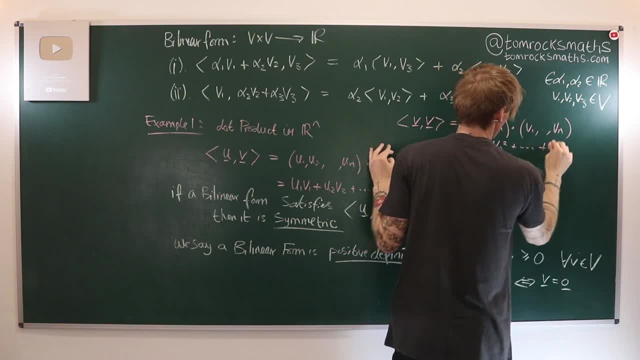 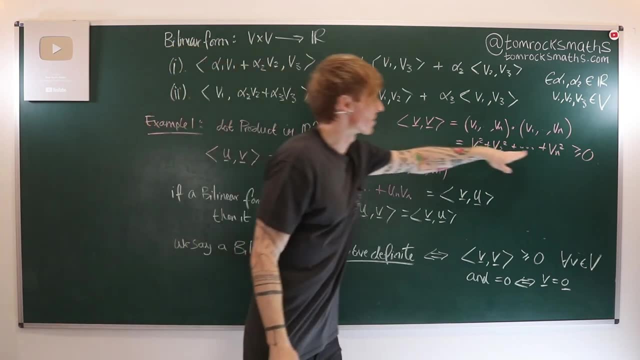 is simply V1 squared plus V2 squared plus dot, dot dot plus VN squared, which we can see is very clearly positive. it's the sum of squares. And then when we Nederland, the only way, this can be zero, because all of these positive pieces are being added. it can only be. 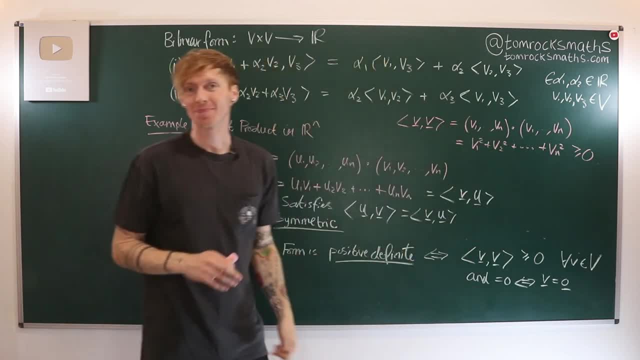 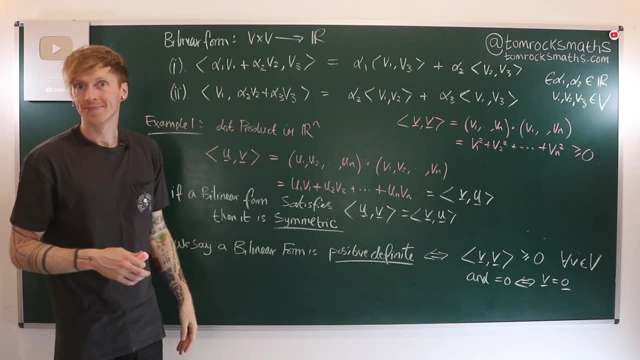 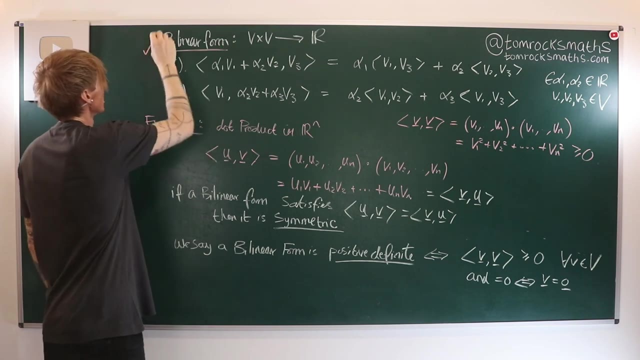 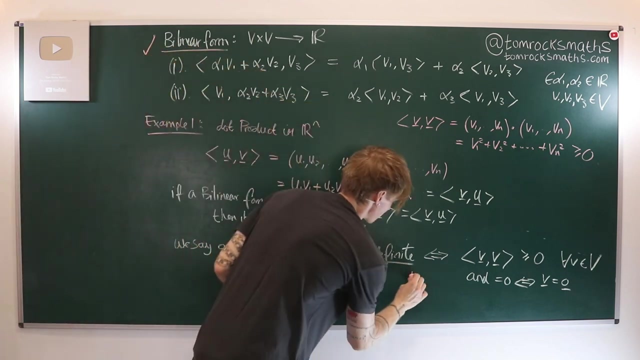 zero. if each individual piece is zero, and if each piece is zero, the original vector was indeed the zero vector in the vector space Rn. So we can in fact conclude that not only is our dot product a bilinear form satisfies, that it's also symmetric and we can say it's positive definite. 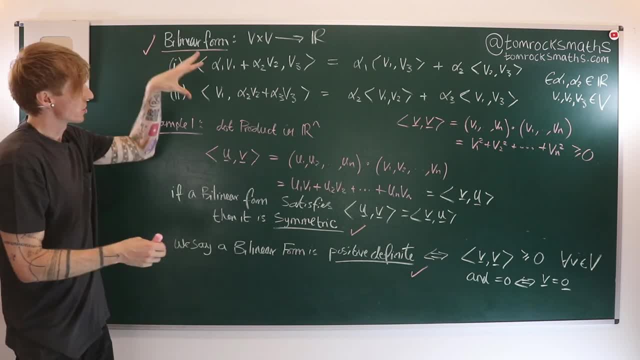 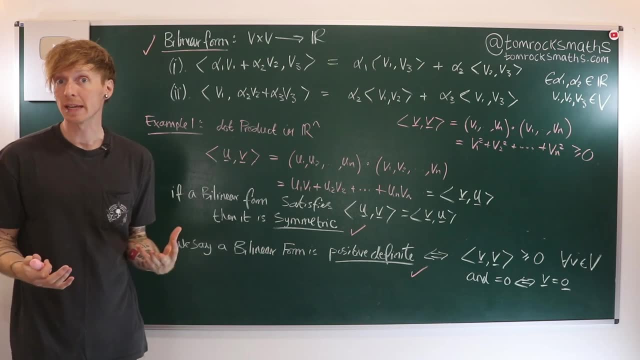 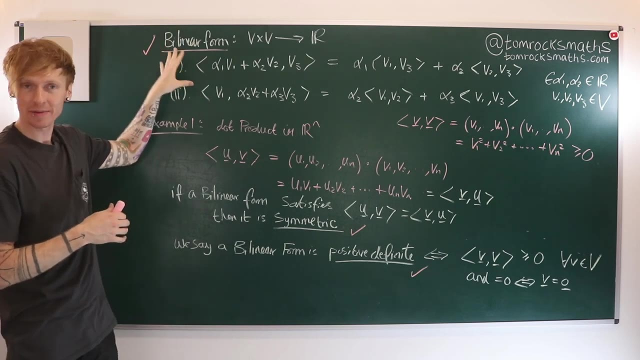 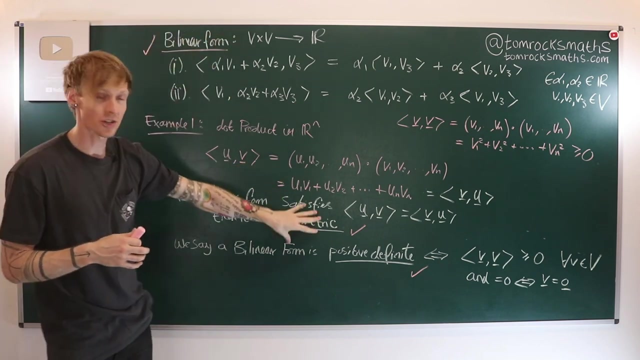 And this allows us to conclude that the dot product on Rn is in fact a real inner product space. More generally, we call any bilinear form- so any map which satisfies properties one and two is linear in the first and second- Any bilinear form which is also symmetric and positive definite. 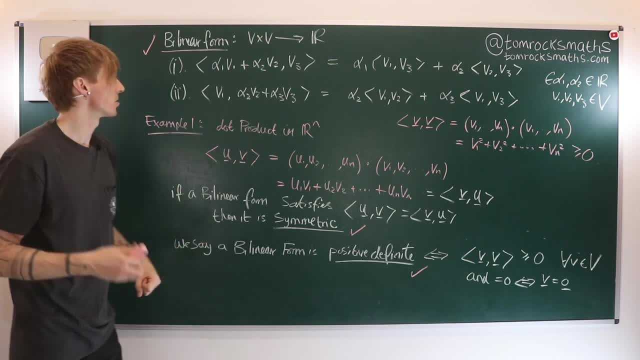 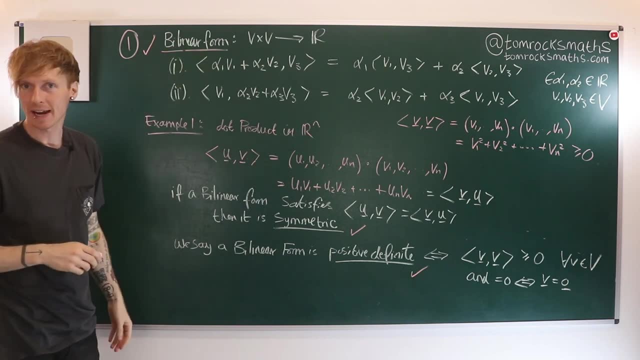 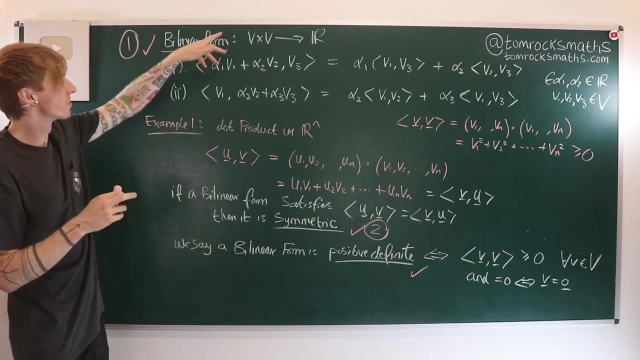 then that is called an inner product. So to be an inner product, you need one, you need a bilinear form satisfying these two properties of linearity. Two, it has to be symmetric, which in fact, as we'll see, removes the need to check both of these as if it's true in one. 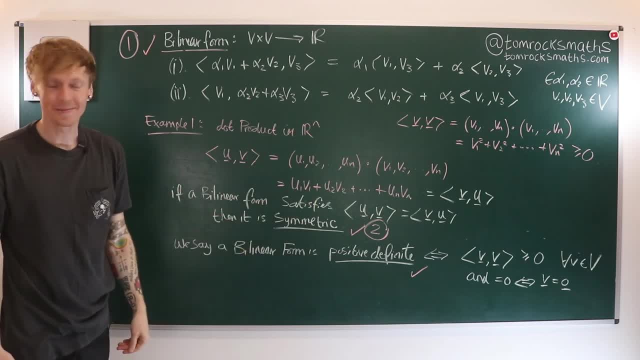 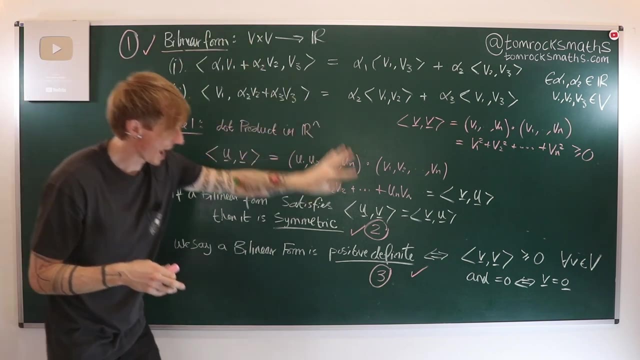 and it's symmetric. you automatically get the second one for free. And third, you need it to be positive definite. So to check whether or not we have an inner product, you have to first show your map is a bilinear form, it's also symmetric and it's positive definite. 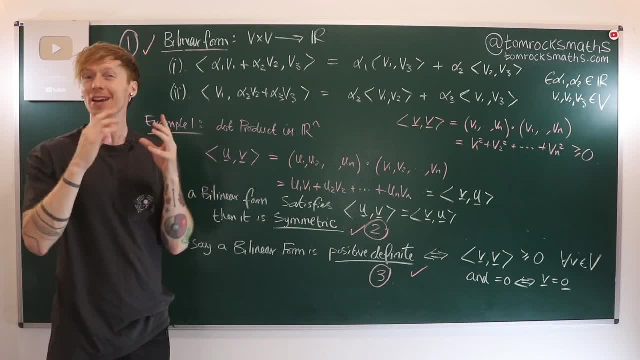 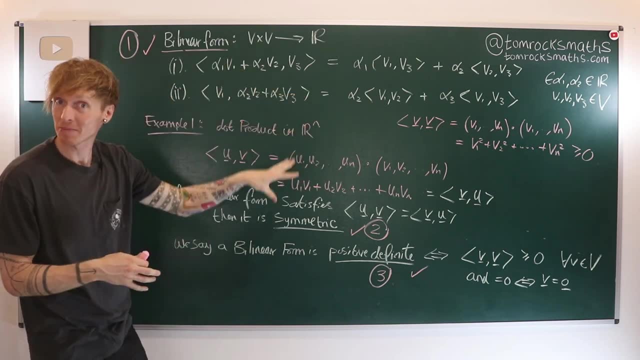 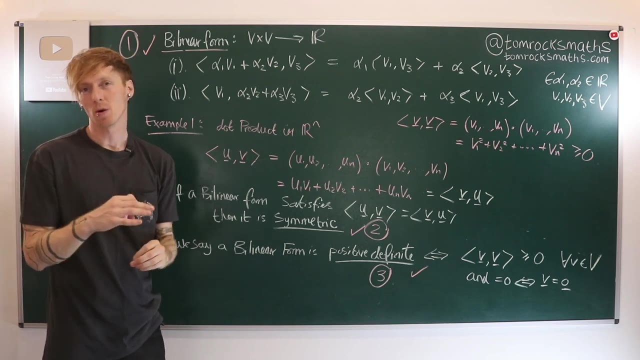 Finally, if you have a real vector space equipped with an inner product, just like here we have our real vector space Rn Equipped with our inner product, the dot product, Real vector space equipped with an inner product- then that is what we call the inner product space. 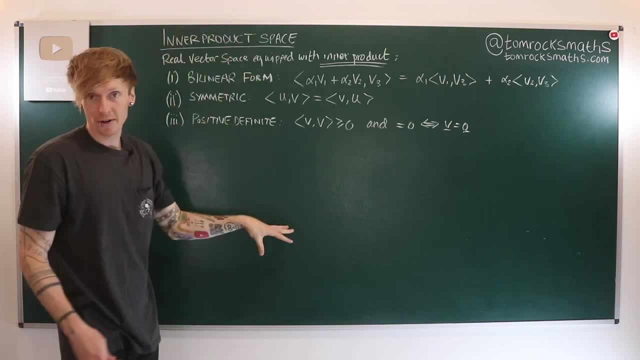 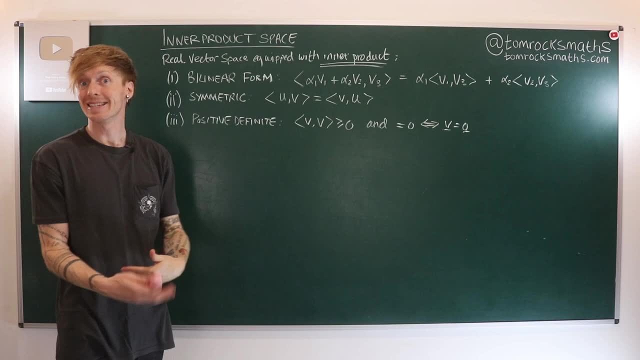 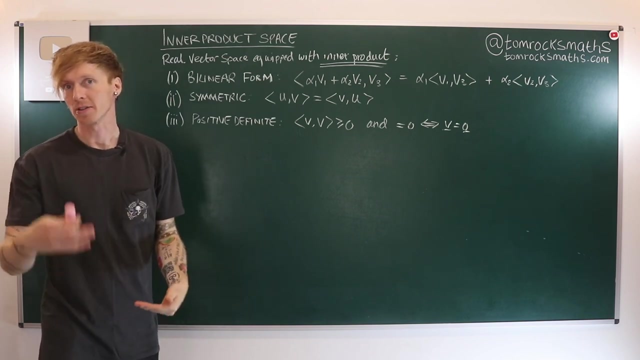 And we've just seen with our example that the dot product on the vector space Rn- so n-dimensional vectors- satisfies all three properties. it is indeed a real vector space and therefore our first example of an inner product space is the dot product on Rn. 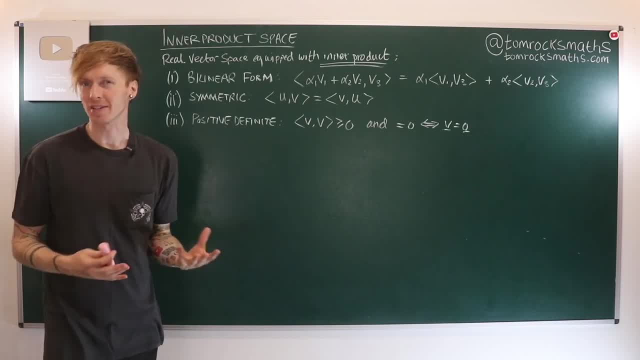 Our second example is going to come from a completely different vector space, and here, in fact, we're going to be talking about functions and, in particular, polynomials within the polynomial vector space. When working with polynomials, we actually define the inner product using an integral, and this may seem vaguely abstract or possibly a little bit random at this point, but 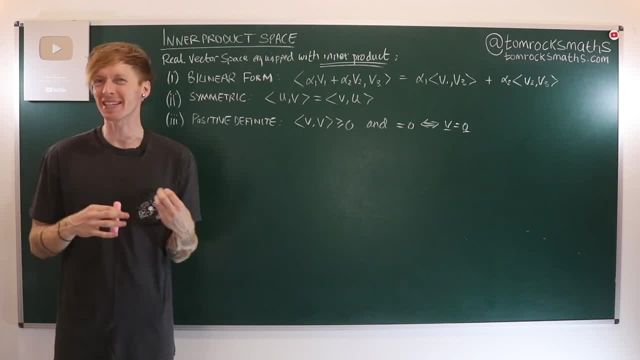 if you have studied any physics or any quantum theory in particular, you may actually begin to recognize why we study inner products in this way and why we define inner products of polynomial functions using an integral. To start, we're going to look at a very simple inner product, which is 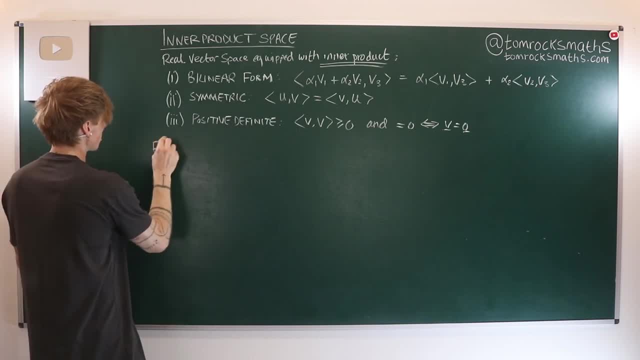 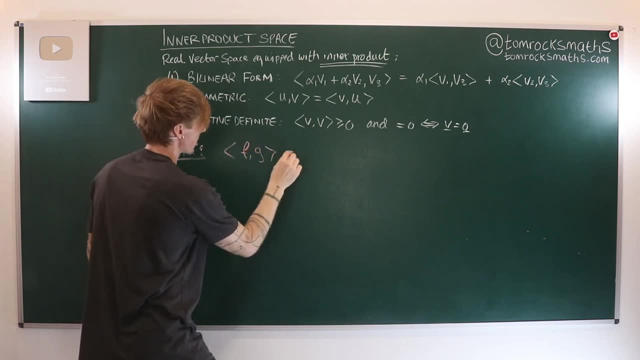 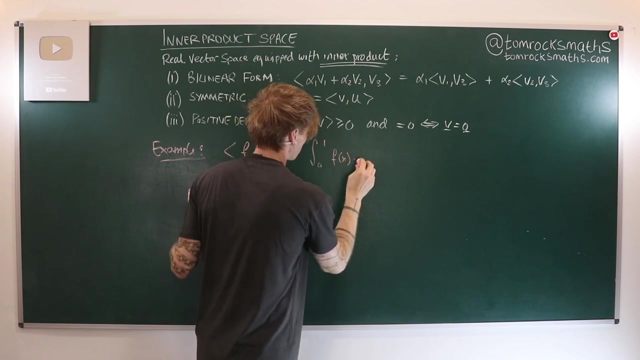 defined as follows. We are going to say that the inner product between two polynomial functions, f and g, is going to be given by the integral from 0 to 1 of f of x multiplied by g of x. Of course we're doing the integral there with respect to x. 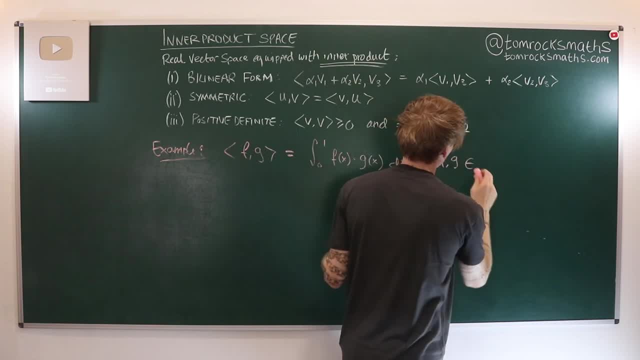 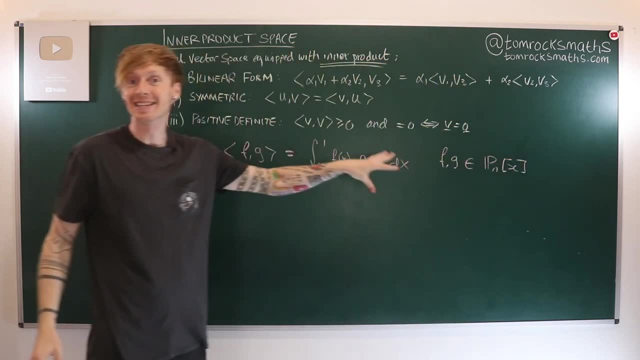 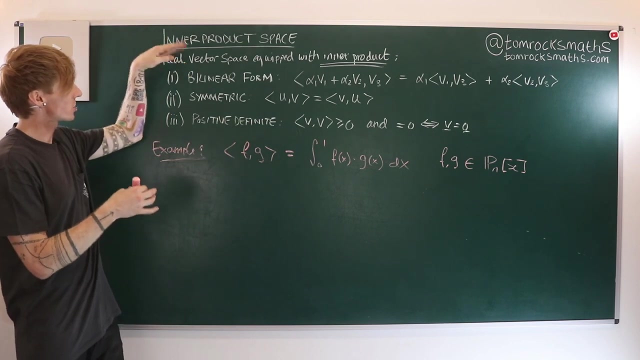 This is going to be where f and g belong to our polynomial of degree n space of x, which we've seen before is indeed a vector space. Of course, we need to check that this is indeed an product, which means checking that it satisfies our three properties. So I'm going to start with. 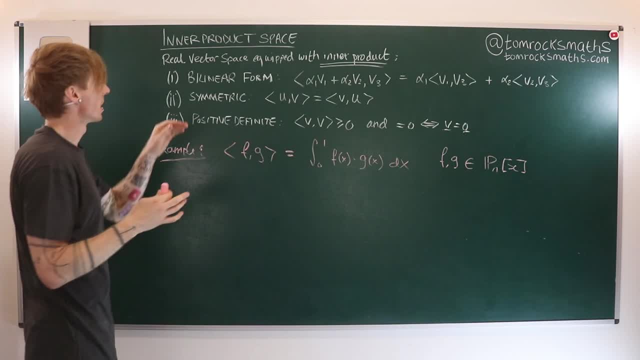 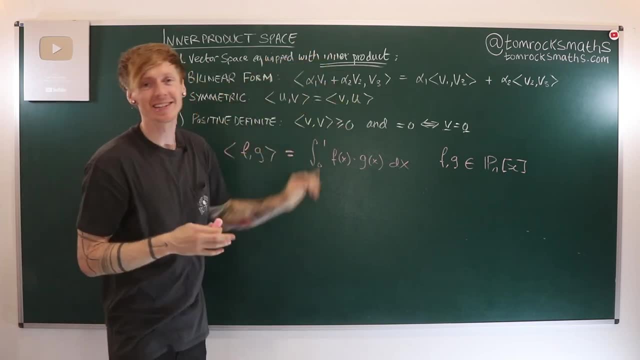 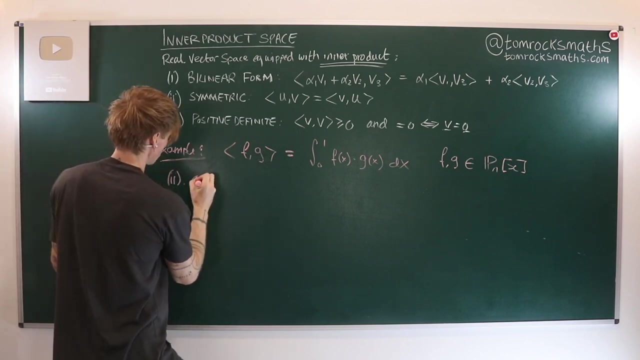 symmetric because, as I've hinted at several times now, once we have symmetric we only need it to be linear in one position, because then, by symmetry, the second linearity actually will follow. So if we consider trying to show that it's symmetric, so number two: 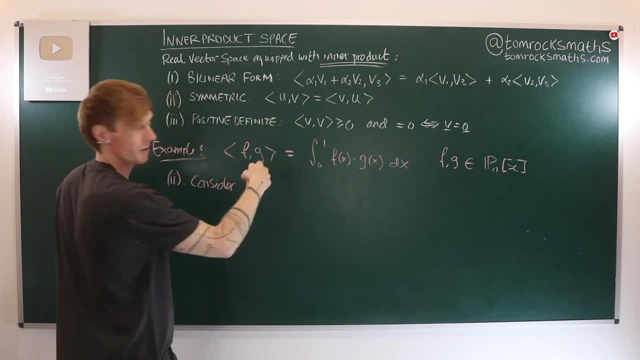 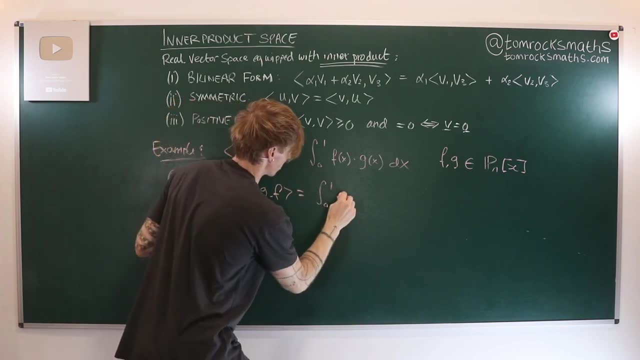 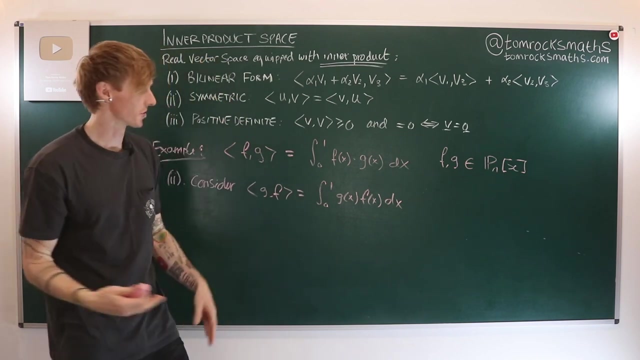 and if we consider so, fg is defined like so, and now I consider gf in a product which is the integral from 0 to 1 of g, of x times f, of x, dx. then by the properties of integrals, we can see: 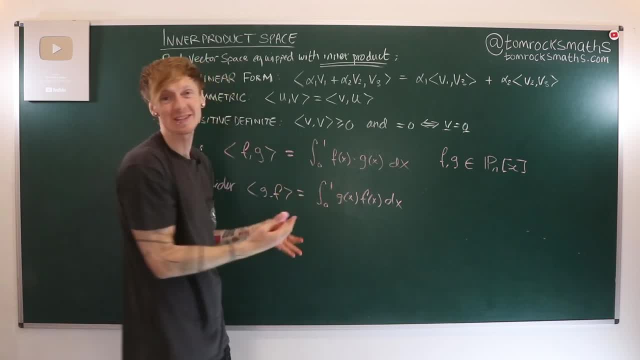 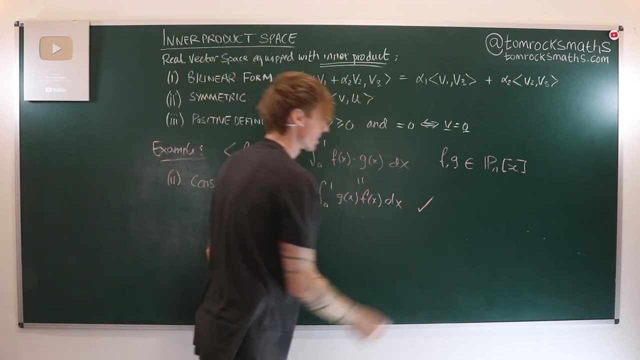 that these are very clearly the same. we can multiply our functions in any order and we should get the same answer. Well, we will get the same answer, So these are equal. so we can say: symmetry is going to be the same and we can multiply our functions in any order and we should get the 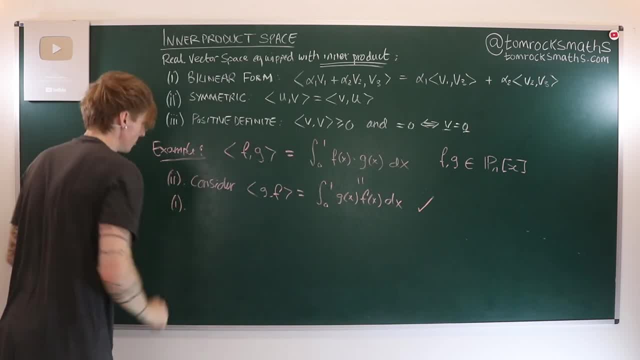 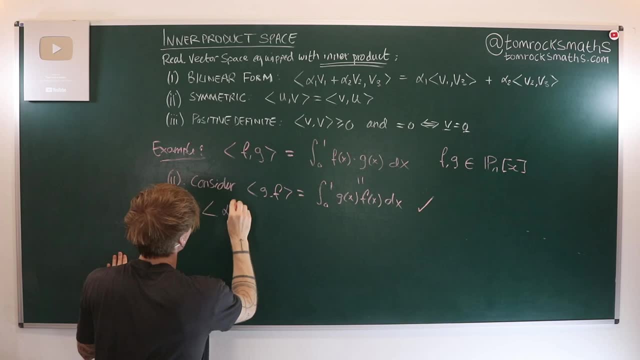 whole. Now linearity by linear form again. now we can just consider it in, let's say, the first position and look at alpha f1 plus alpha 1, f1 plus alpha 2, f2 comma g, So again by the definition. 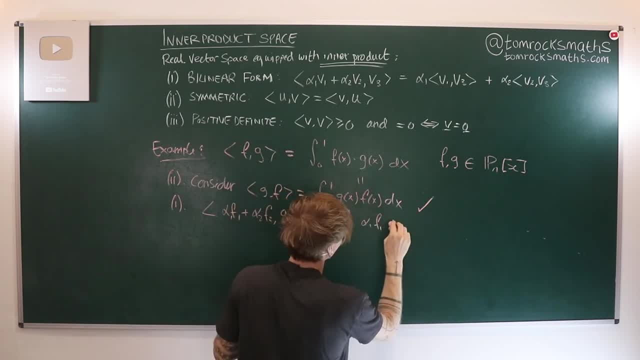 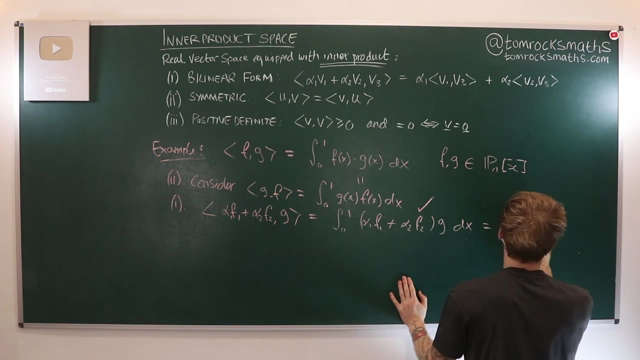 that's 0 to 1 of alpha 1- f1 plus alpha 2- f2, multiplied by g dx. but of course that's going to split up into two pieces. so we can say: that is pull out the alpha 1, we've got 0 to 1 of f1- g dx. and then we've got plus alpha 2 integral, 0 to 1 of f2- g dx. 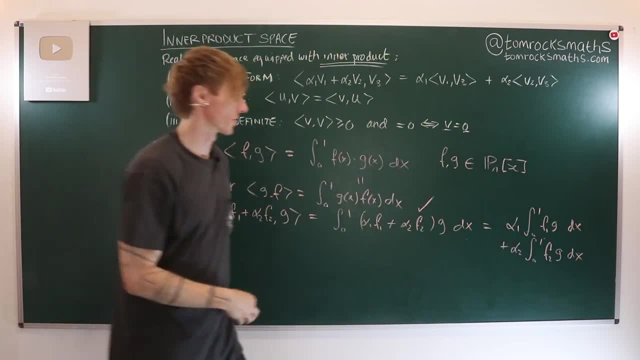 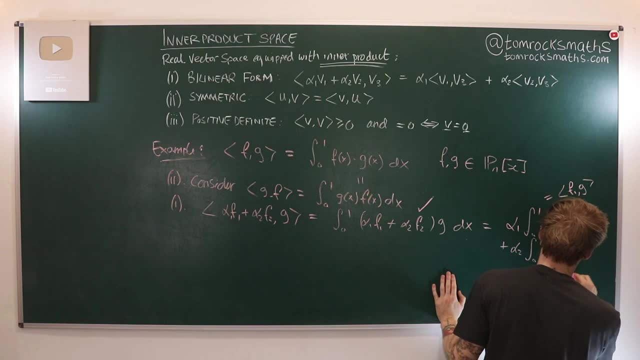 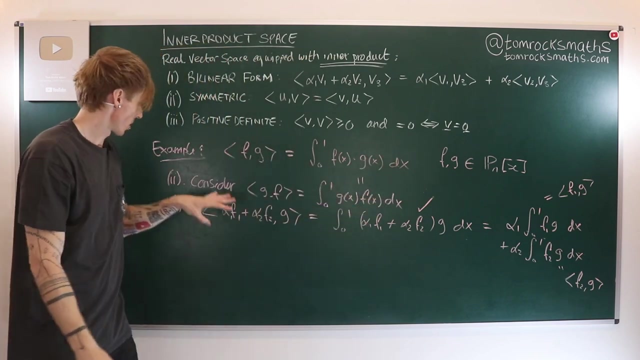 and now, hopefully you can see, these two individual integrals are going to be our two pieces. So this is f1, g and this one here is f2 and g in our inner product definition as the integral. So one is satisfied, we've got a. 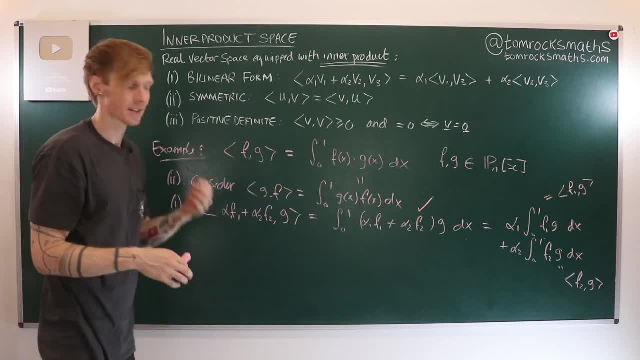 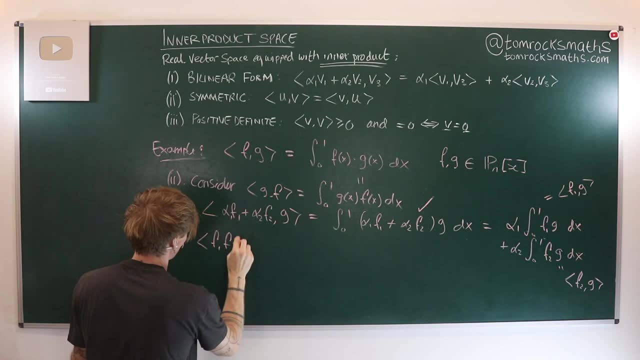 bilinear form. it's also symmetric, so that just leaves us with positive definite. So for number three, we want to consider f with itself. so the inner product of f with f by our definition is 0 to 1 of f squared dx. Now we have a square function. 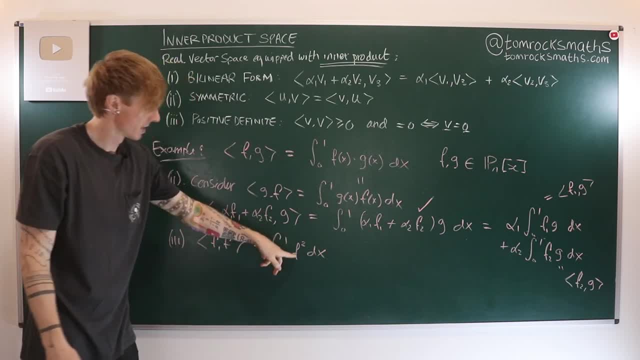 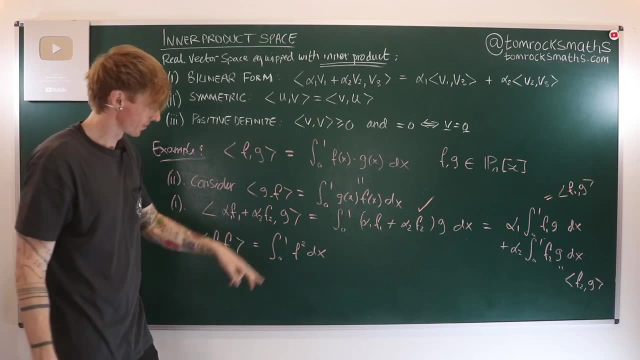 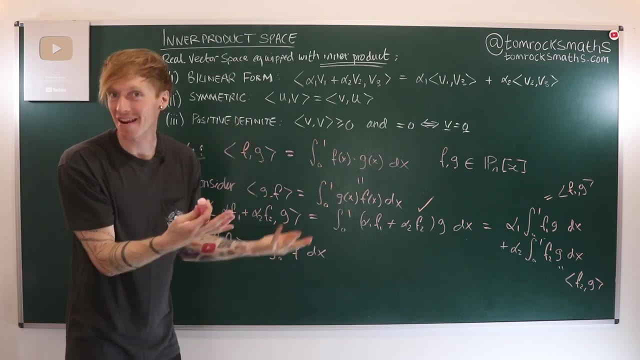 another square polynomial function. So this, the integrand, is always positive because, again, it's a function which has been squared. So we have the integral of something that's always positive, and of course the integral represents the area under a positive curve. so 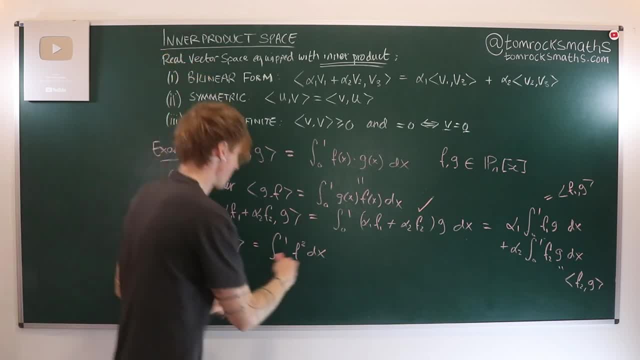 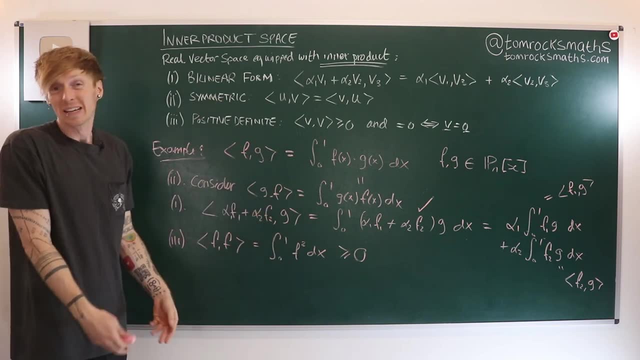 therefore, this will always be greater than or equal to zero as well. So again, properties of integrand say that this is always positive, because we're integrating certain signs of inner product. there is always positive among явly nodes, something that's always positive, and in fact, the only way it can be zero is if the function is. 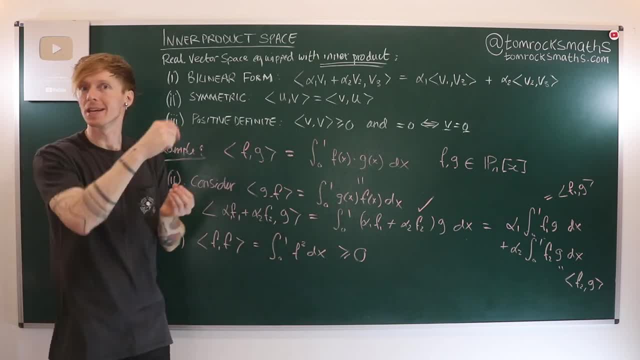 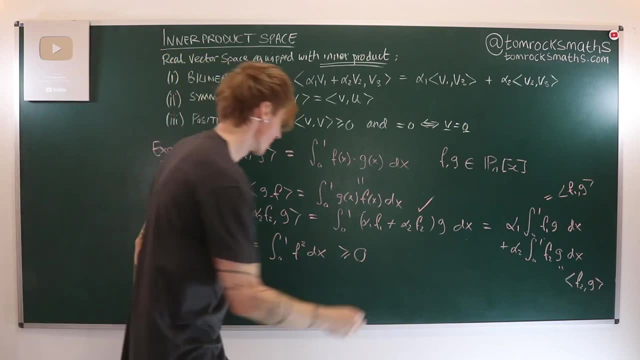 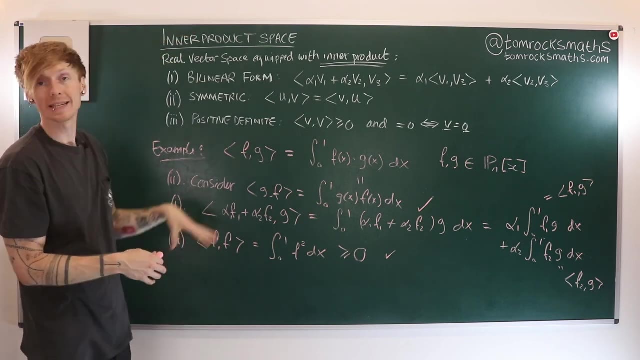 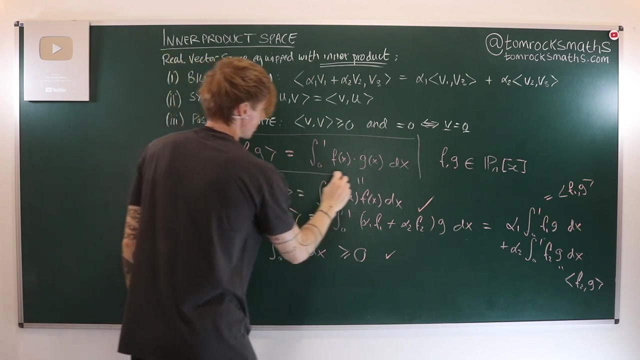 everywhere zero, because if we have a non-zero bump anywhere, then we're going to have a non-zero area under that bump. so it will indeed satisfy positive, definite and therefore we can conclude: all three properties hold and thus the integral inner product as defined here is indeed an inner product. 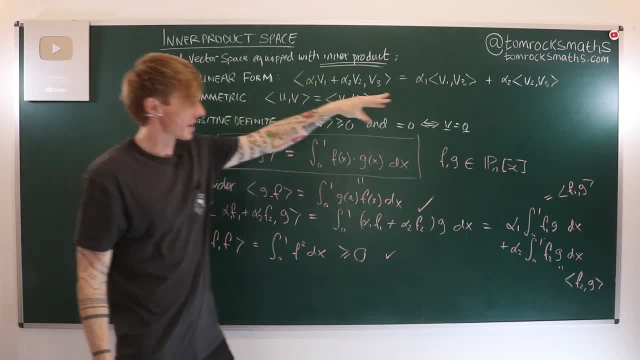 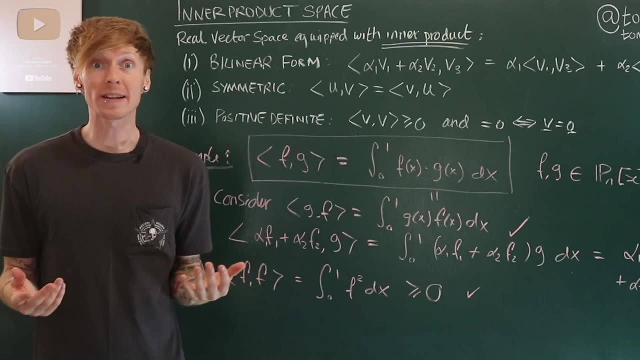 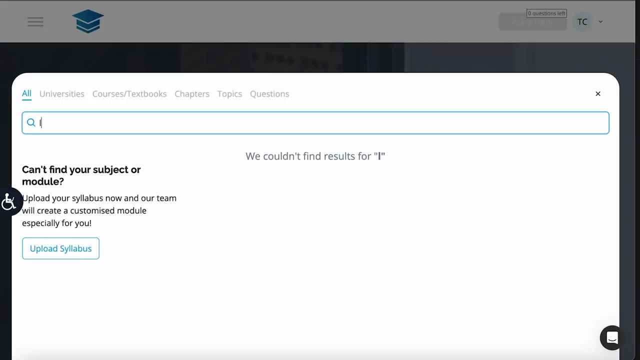 we can now say that and because we're taking real coefficient polynomials, we can in fact say that this is an inner product space. For more examples, including others involving the polynomial space, be sure to check out ProPrep, an online resource which provides video tutorials for 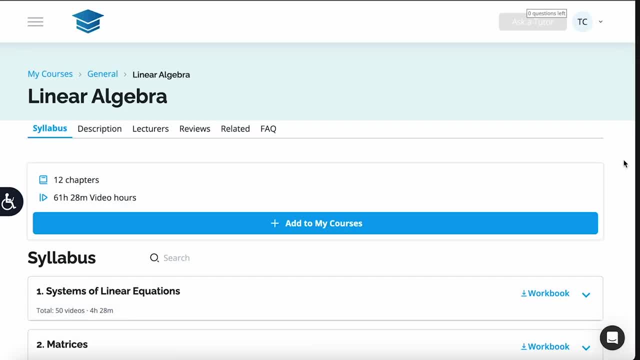 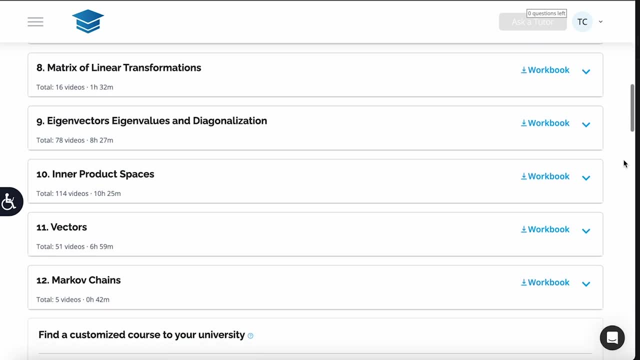 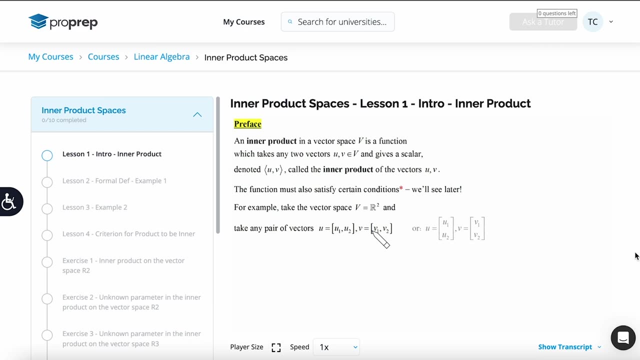 anyone looking to learn how to do that, to improve their skills in stem based subjects. As with all topics in the Oxford linear algebra series, ProPrep offers a number of video lectures to help to solidify what you've seen in this video, as well as numerous exercises, each with their own video solution, Beginning with the standard. 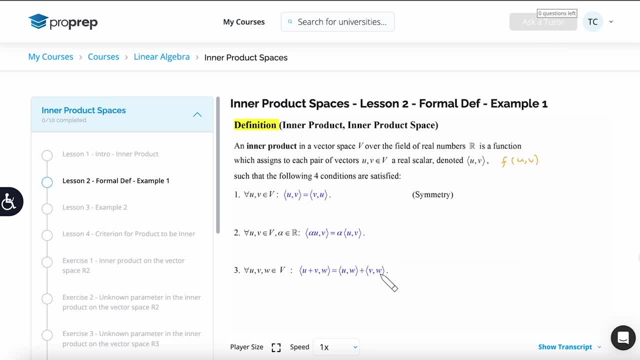 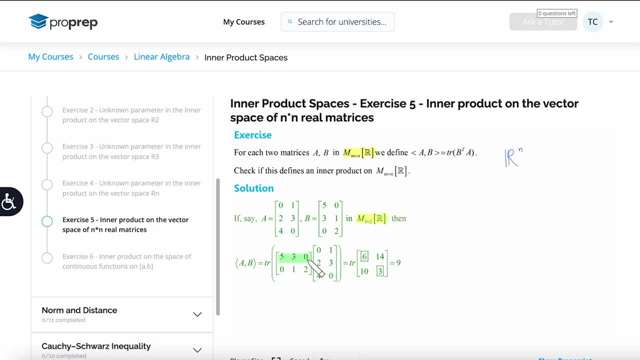 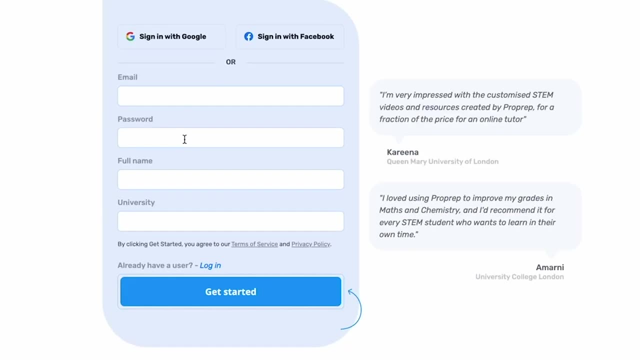 vector spaces of R2 and R3. there are further examples in Rn, more from the polynomial space and even an inner product defined over the vector space of matrices. Click the link in the description to see more videos on this topic. Click the link in the video description below to sign up for your 30-day free trial. courtesy of Tom Rock's maths. 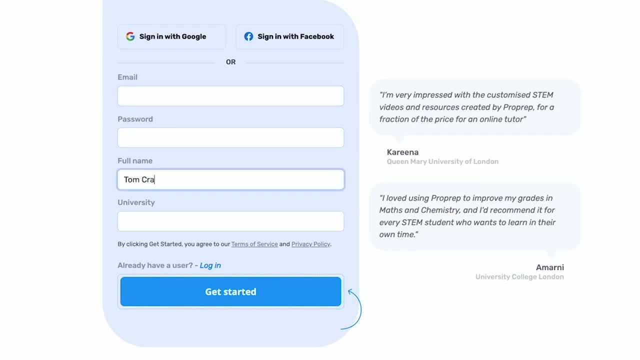 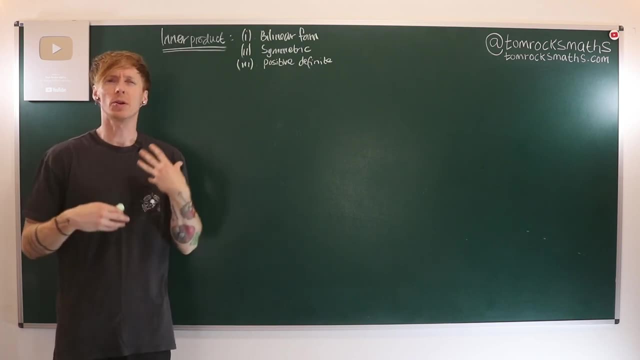 and see just how much ProPrep can help to improve your learning When working in an inner product space. there's a very nice way to construct a basis using what is called an orthonormal set. Here's the definition. So an orthonormal set is a set of vectors, let's call them v1 to vn belonging 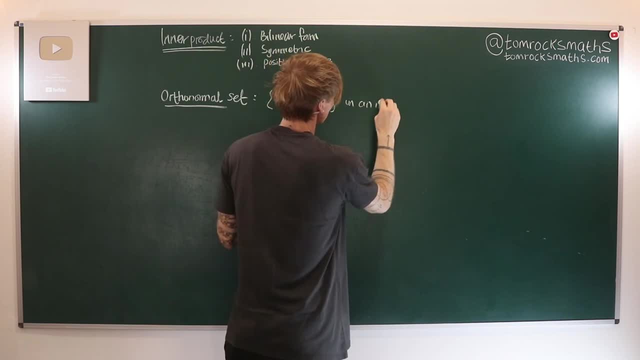 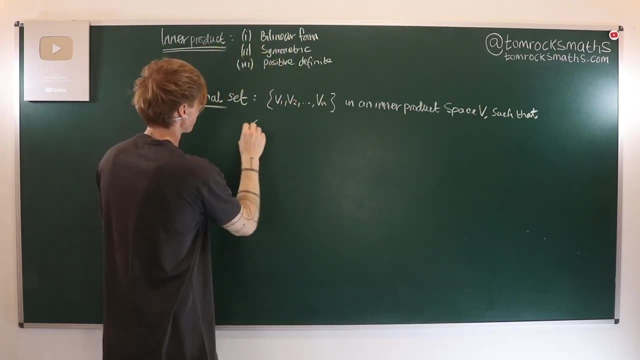 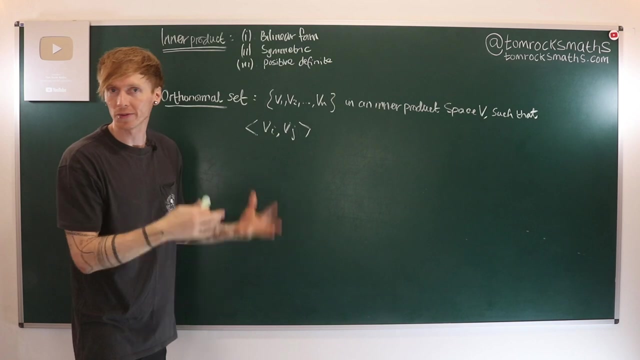 to in an inner product space, in an inner product space, v, such that when you take the inner product between any of them, so you take the inner product of vi with v, j, where i and j can range from one through to n, then the answer here is what we call delta ij, the delta function, which is defined to be one. 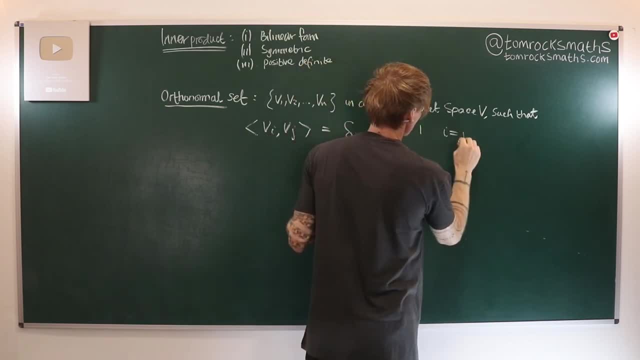 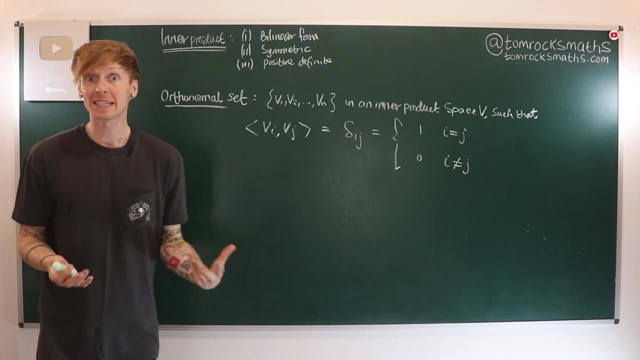 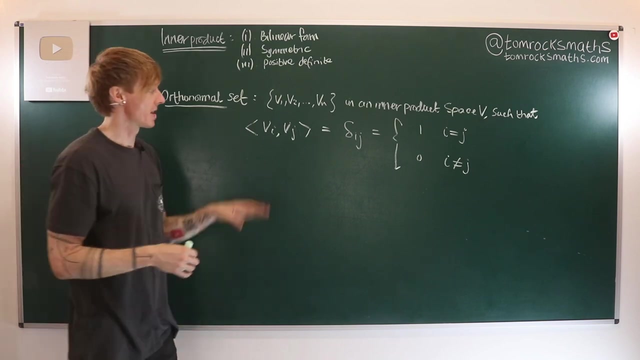 if i Vallahi split, their order by some reason is equal to j and 0 if i is not equal to j. So what this is saying is that if you take the inner product between any two vectors in your orthonormal set, then you: 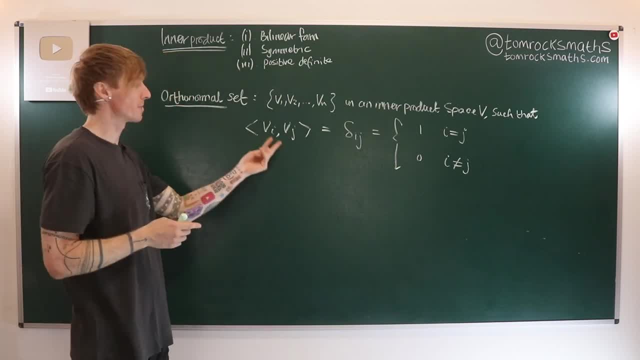 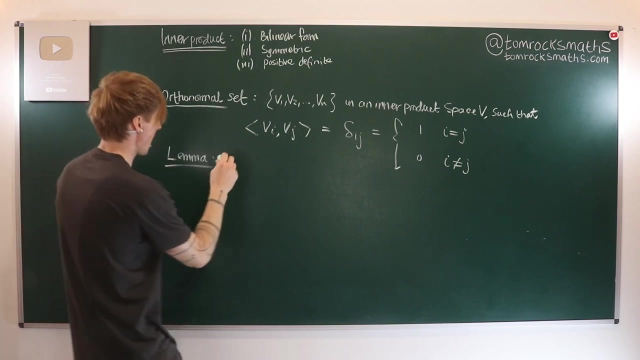 will get 0, unless they happen to be exactly the same vector, in which case you will just get 1.. Armed with this definition, we can now actually prove the following lemma, which relates back to what I was saying about this being helpful for constructing a basis. So the lemma says the following: For v1 to vn. 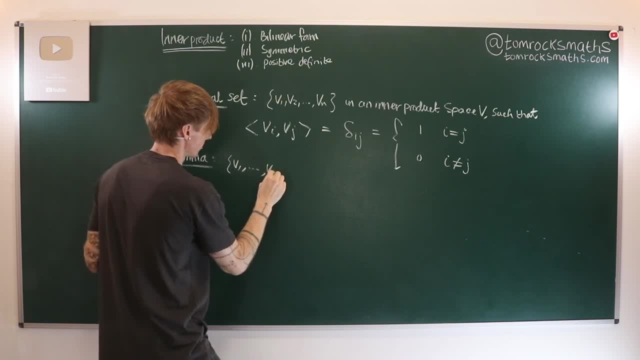 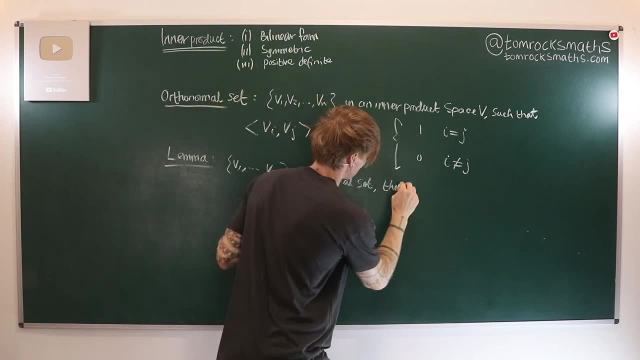 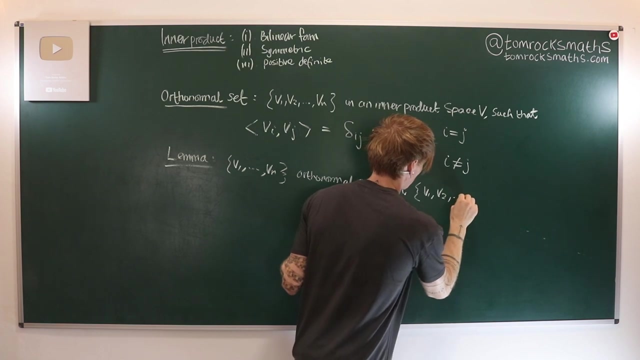 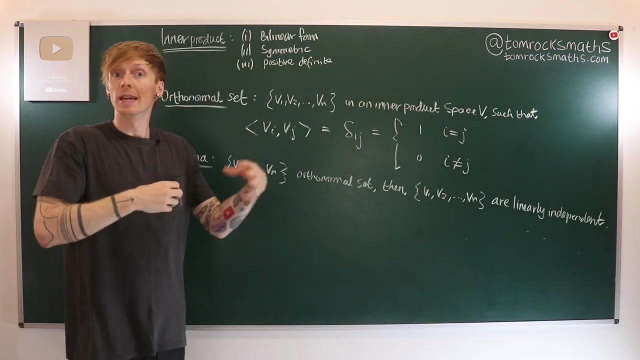 an orthonormal set, which again means they fit this definition- orthonormal set- then in fact we can conclude that v1 to vn are linearly independent sets. So v1 up to vn are linearly independent. So of course, in order for a set to be a basis, it has to be both. 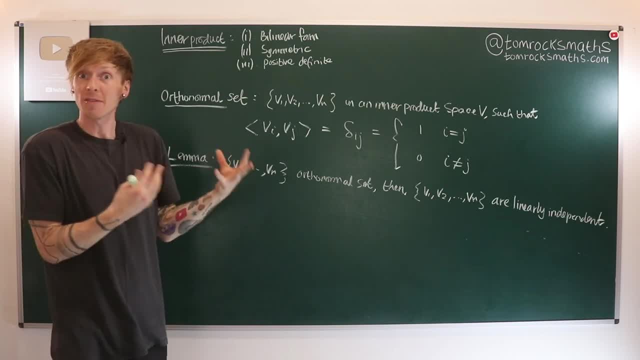 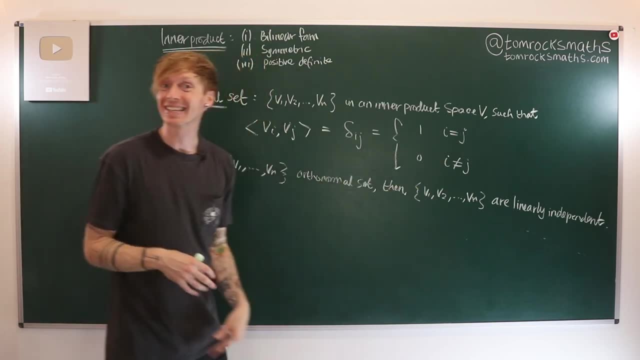 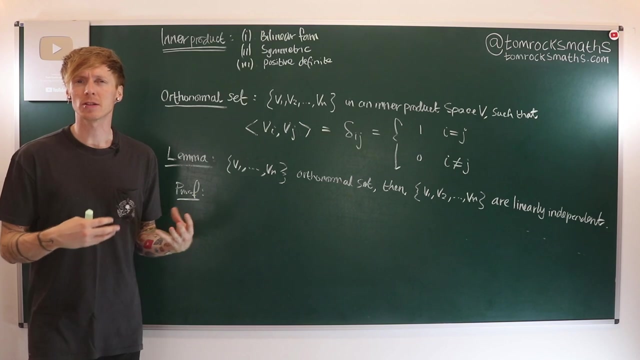 spanning and linearly independent. So if we have an orthonormal set within our inner product space, this lemma is telling us that we actually have a linearly independent set. So let's prove it Now. whenever we consider linear independence or we have to show a set is linearly independent, 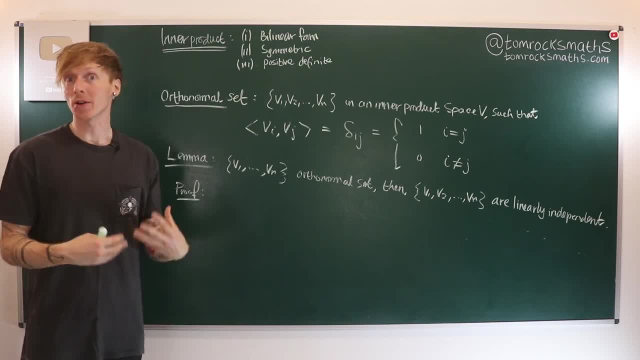 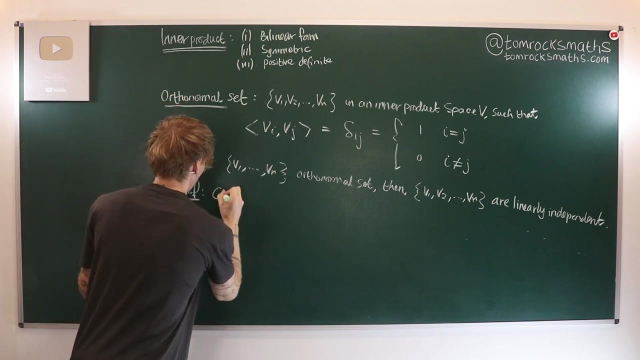 there is a particularly helpful way of trying to show that property, which is to consider a linear combination of those elements and argue that all of the coefficients must be zero if the total combination is going to be zero. So we start following that. So we say: consider: 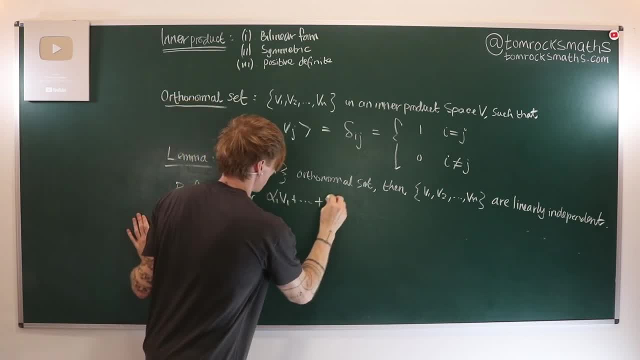 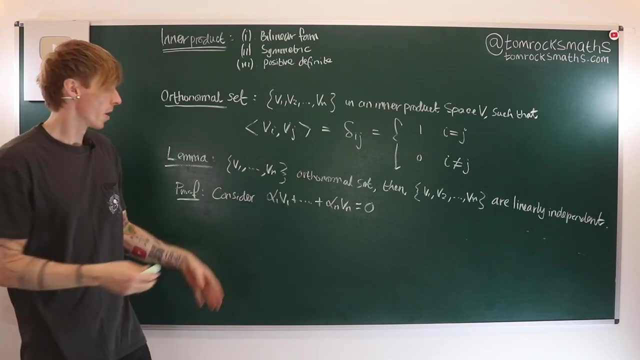 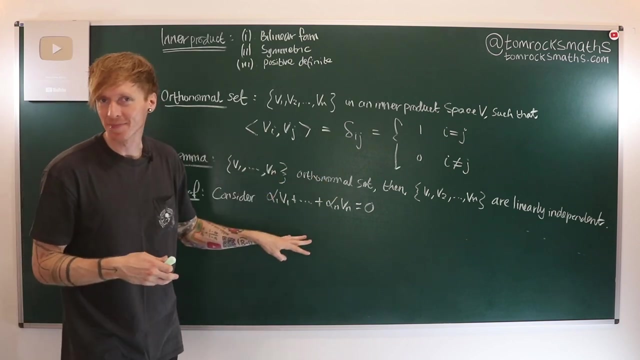 alpha one v one plus dot, dot, dot, plus alpha n v, n, and we suppose we can create such a combination to be equal to zero, where some of these alphas could indeed be zero. but our goal is to show that, in fact, the only way this can hold is if all of the alphas are zero And if we can show that. 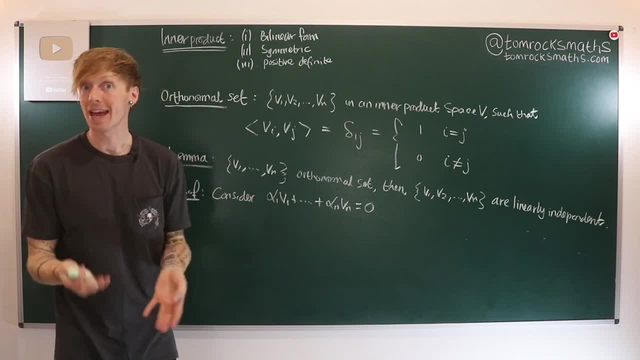 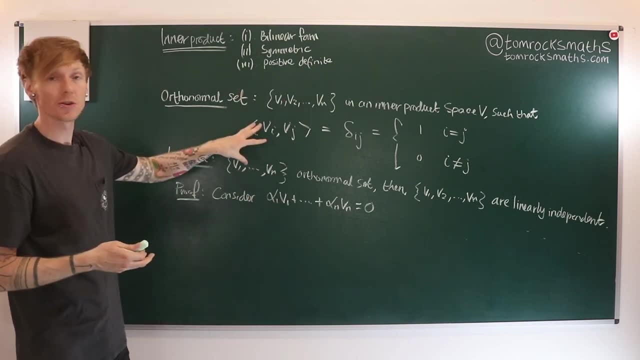 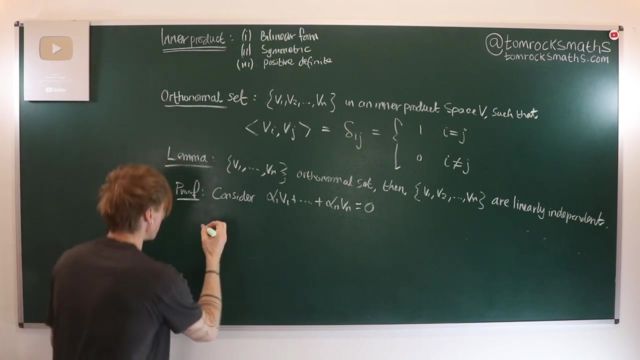 if we can show that alpha i is not for all i, then we can conclude that we have linear independence. So we clearly need to use orthonormality and we're obviously going to have to take some inner products. So what we do is we start by saying, well, zero is actually equal to the inner product of 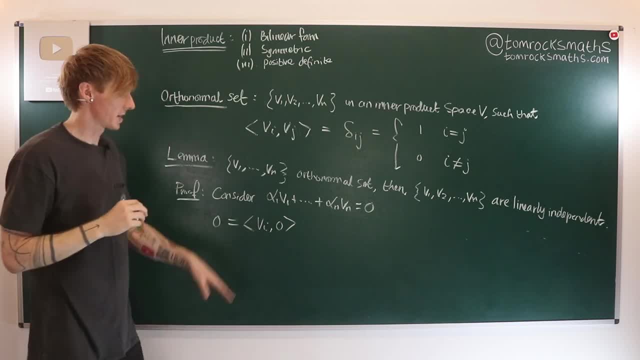 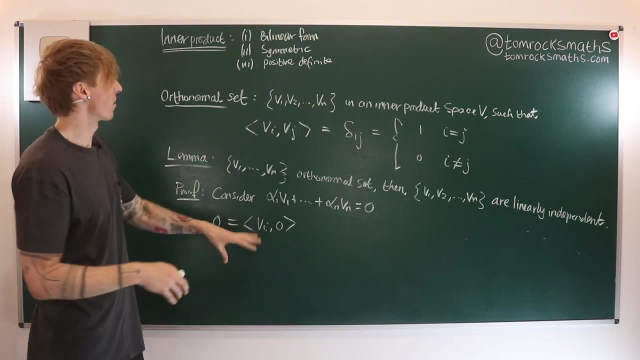 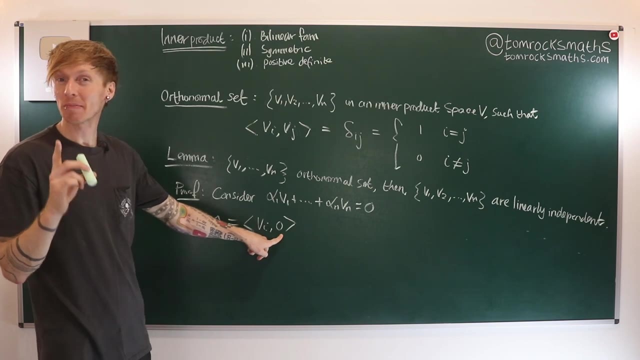 v i with zero, because if we take the inner product of anything with zero, we're going to get zero. That's kind of how inner products work and that would follow from these properties up here. But now we can replace the zero inside our inner product with this combination here, which of course is zero. 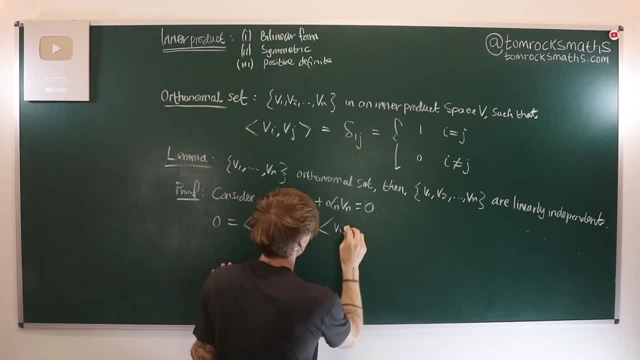 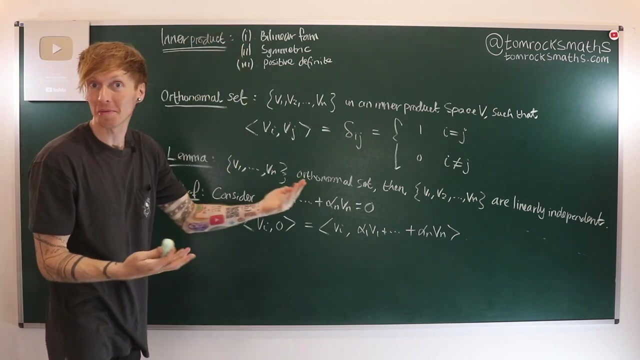 So we can say: well, actually this is the same as v, i comma, alpha one, v one plus dot, dot, dot plus alpha n, v, n. Now we can explicitly use linearity. So property one it's a bilinear form because it's in a product. 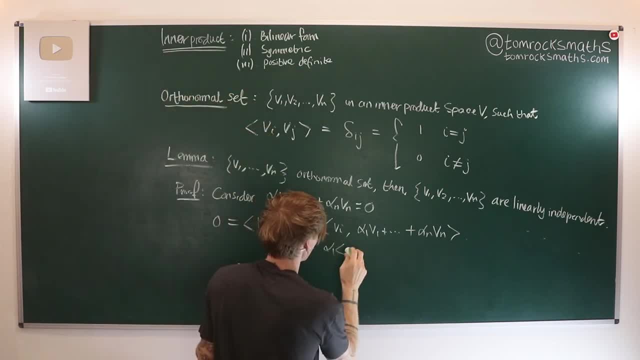 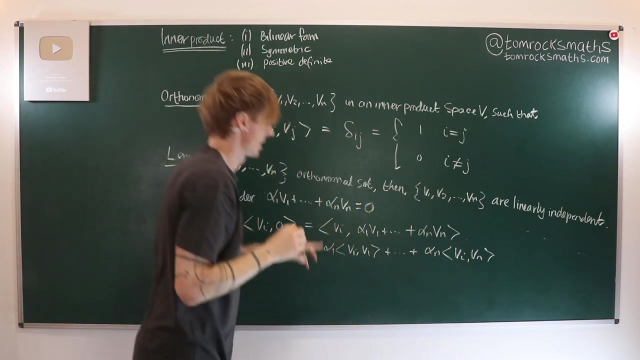 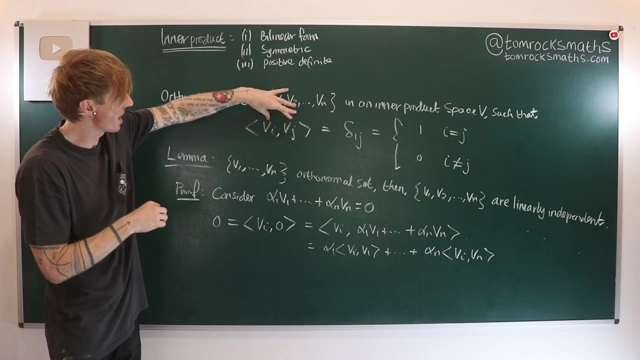 So we split this up now, we pull out alpha one and then we've got v? i comma v one plus dot, dot, dot plus alpha n. v i comma v n. Now is where we use orthonormality. So up here we see that we have a pair of our vectors and it 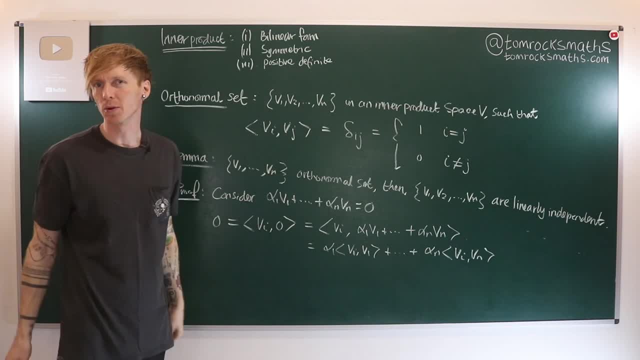 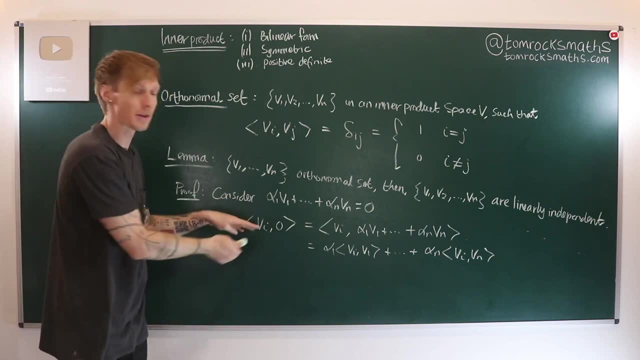 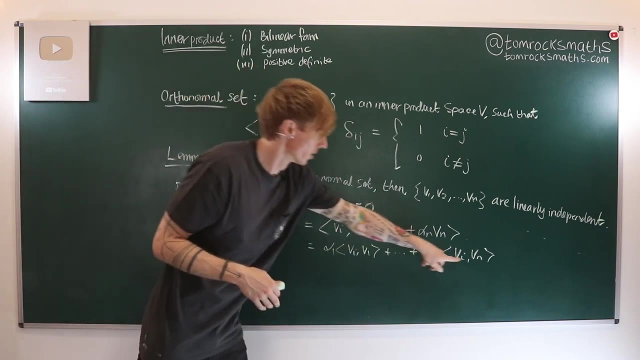 tells us we can only get zero or one. That is the property of being an orthonormal set. Now down here we have a pair of pairs. Now i is arbitrary. we could let i be one through to n, and that's kind of what we're going to do. But whatever value we have here, we know from this property of 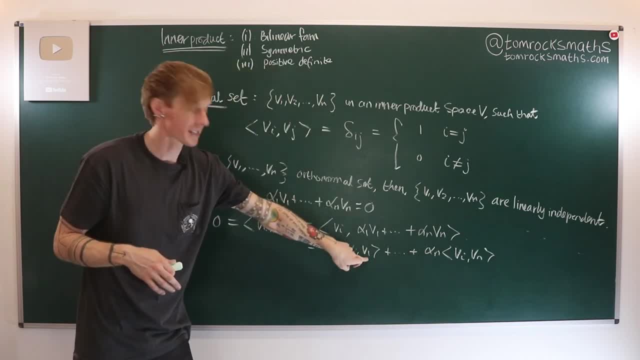 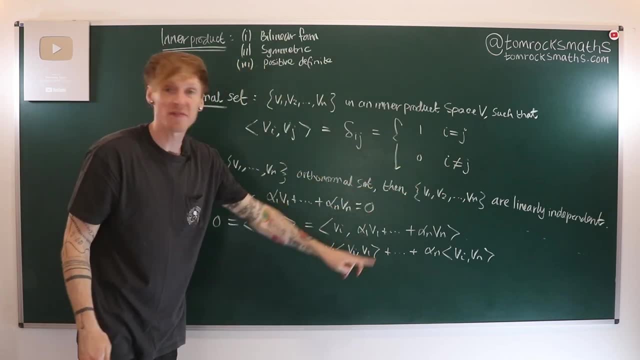 orthonormality that these are all going to be zero unless i is the same as this number. So i and j have to be equal, otherwise we get zero. So we're just literally going to get v- i. So all of these are zero except. 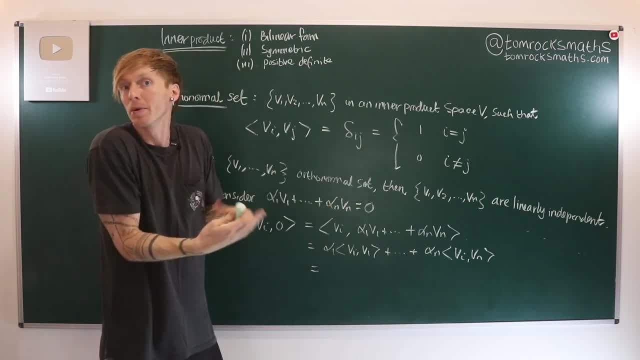 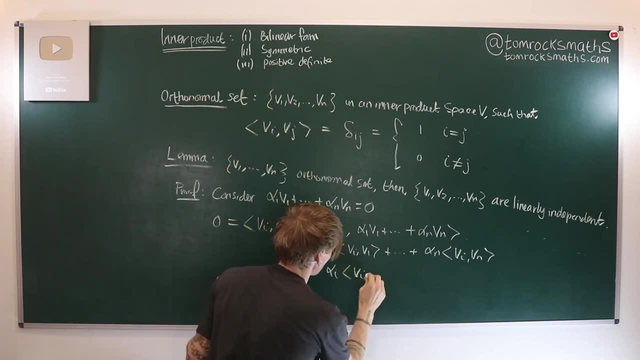 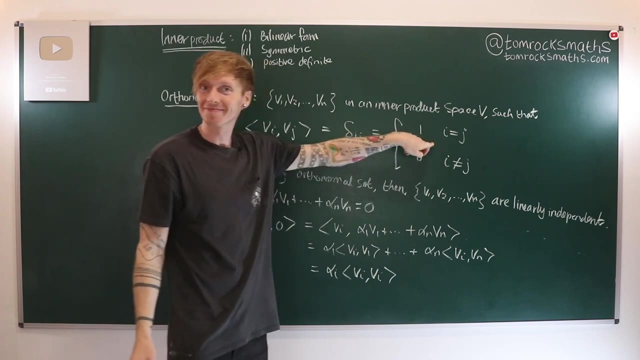 one. as we count up one, two, three, etc. we will hit i at some point. So what we're going to be left with is alpha i, v i, comma v i, But now we have v i, v- i, so they're the same thing, which is one. 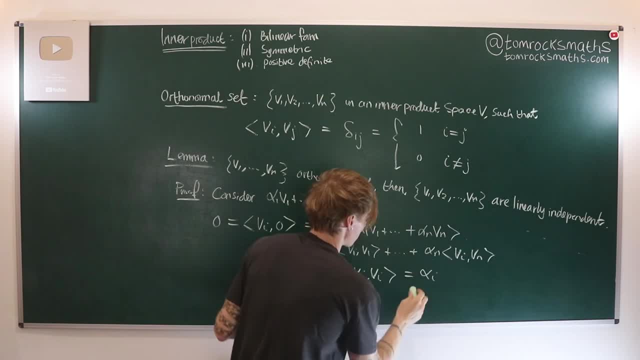 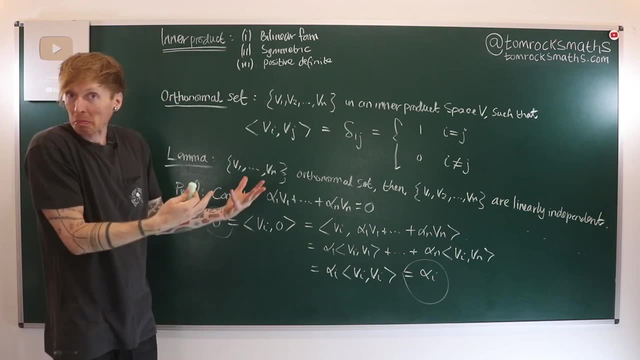 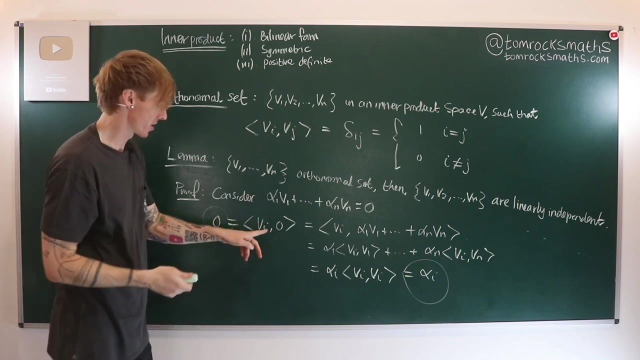 So that's actually just alpha i. So we've got alpha i is equal to zero. And again- and you might want to do this to convince yourself, sort of step by step- this is going to work. I could have taken i to be anything, So i could have been one, and then i would get alpha one v one v one, which is: 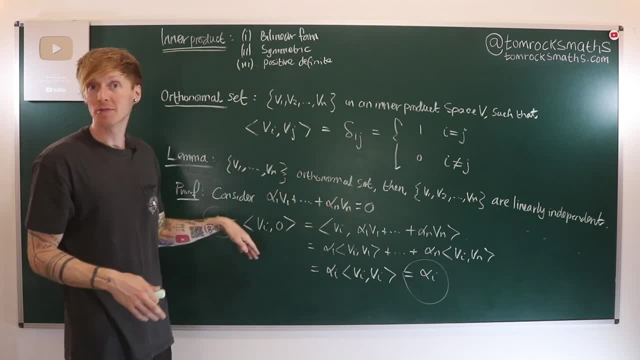 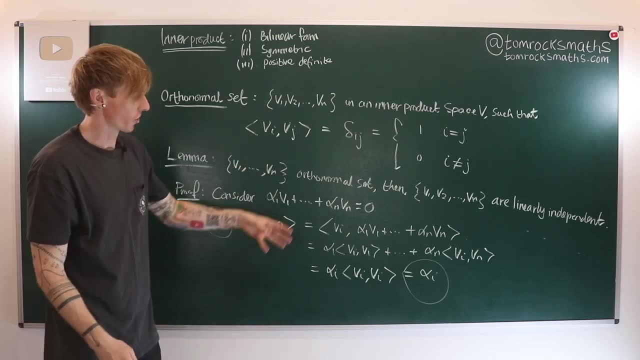 just alpha one, And then i would have got: alpha one is zero. and then i use: i equals two, i equals three, And you can count through each step. there are n steps and you'll show that all of them are zero. Or you can keep it nice and general, as i have here, and realize that i represents an arbitrary. 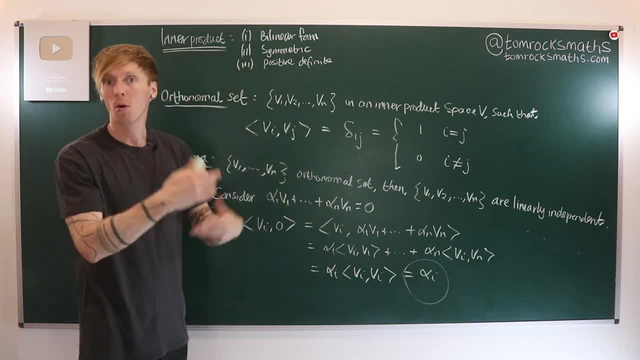 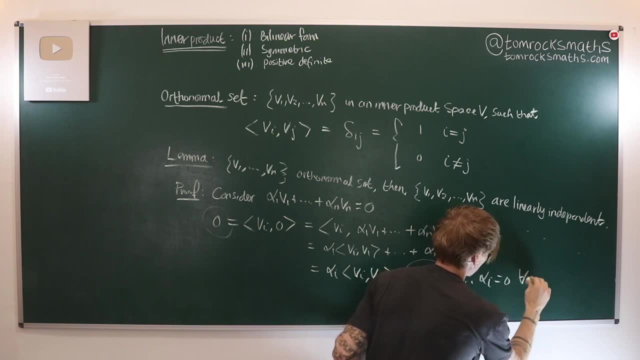 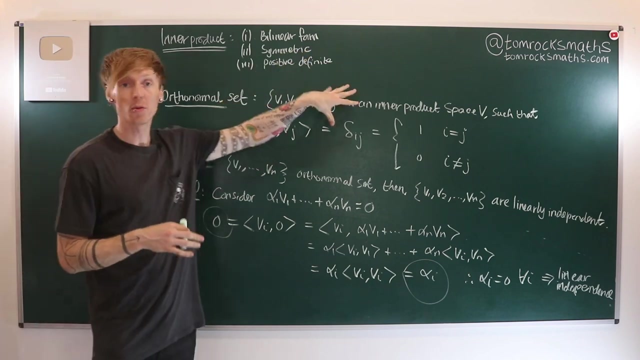 vector and therefore an arbitrary coefficient, We're going to see that all of them are zero. so therefore the alpha i is zero for all i, from one to n, And so that allows us to conclude that we do indeed have linear independence. So now we have linear independence of our orthonormal set. So anytime we have an 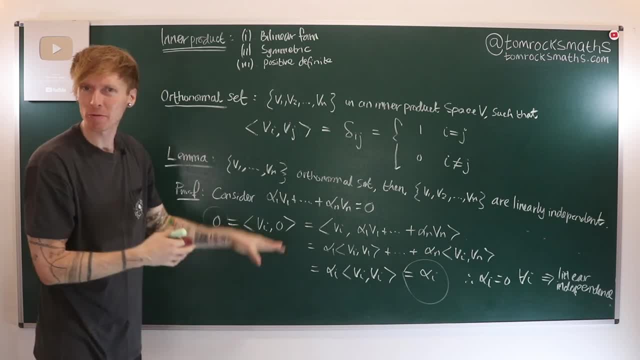 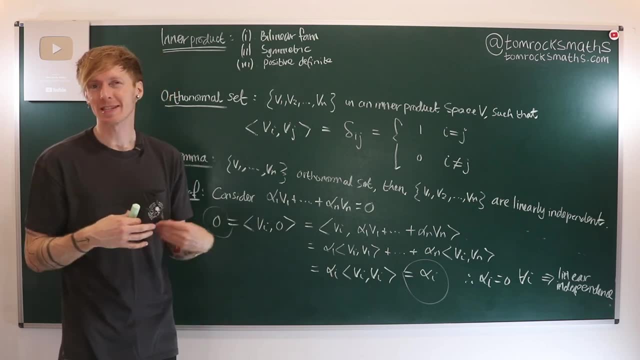 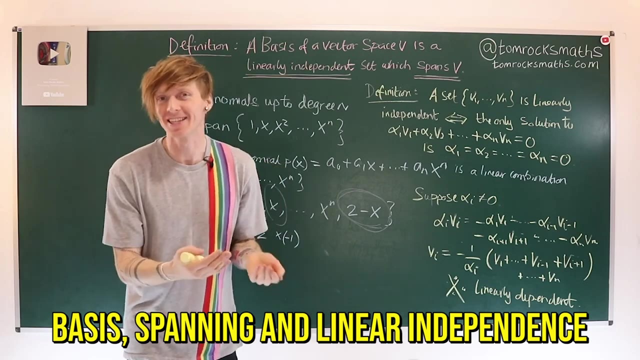 orthonormal set- this lemma has allowed us to show it will always be linearly independent, So the only thing that's missing from it being a basis is for it to be spanning. However we've seen before in the video on linear independence, spanning and basis previously in this series, 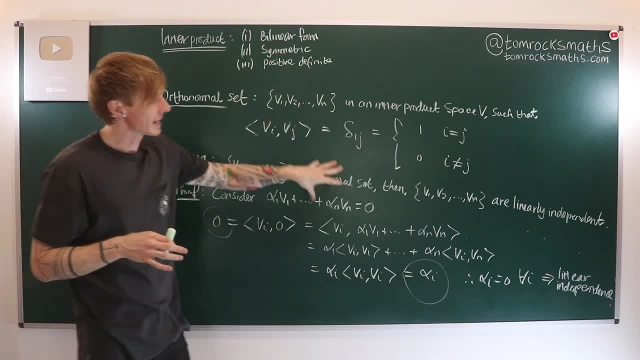 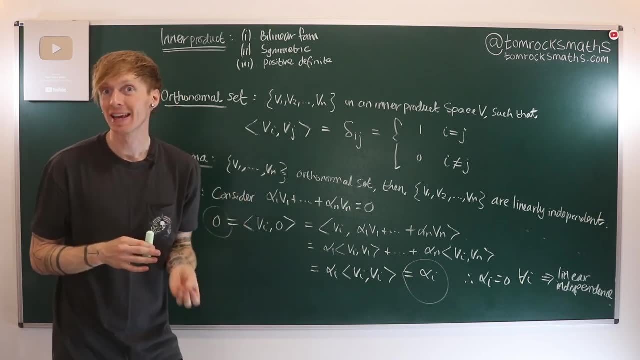 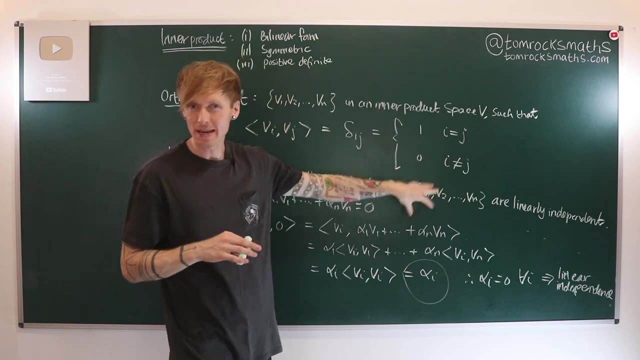 we've seen that if we have a linearly independent set which has the same dimension as the entire vector space, then it is indeed a basis. So any linearly independent set with the same dimension as the whole space will in fact be spanning and therefore will in fact be. 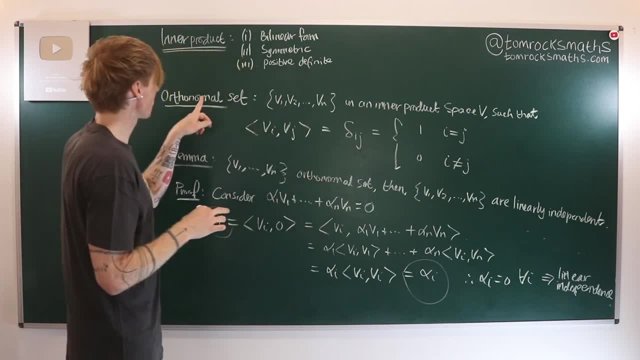 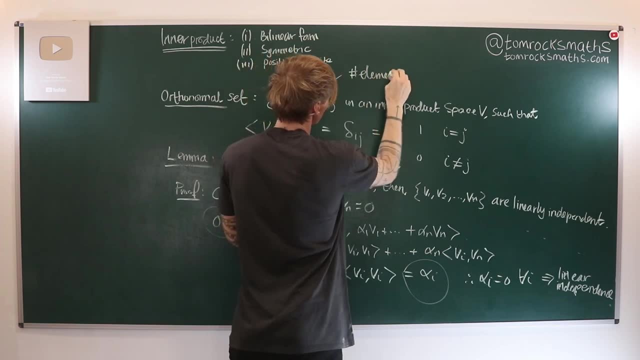 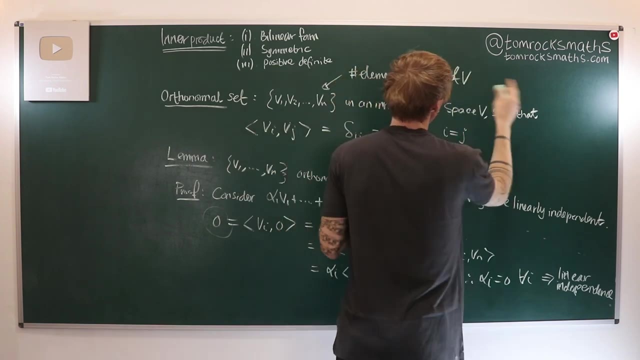 a basis. So what this means here is that if we have an orthonormal set which has the number of elements equal to the dimension of r in this product space, v, then this is actually allows us to conclude that this is indeed going to be. 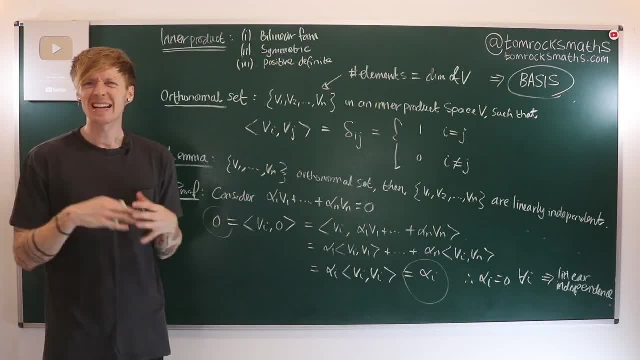 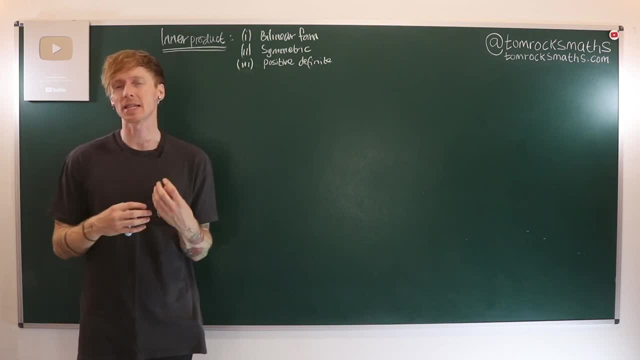 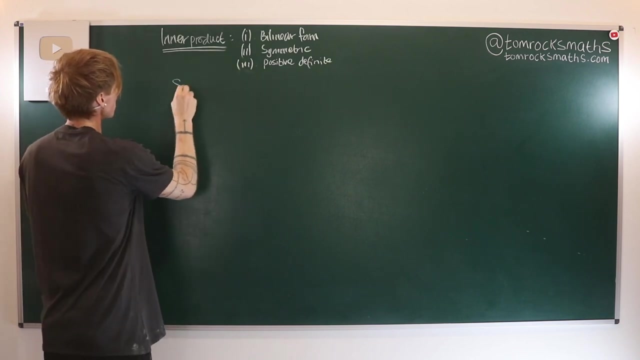 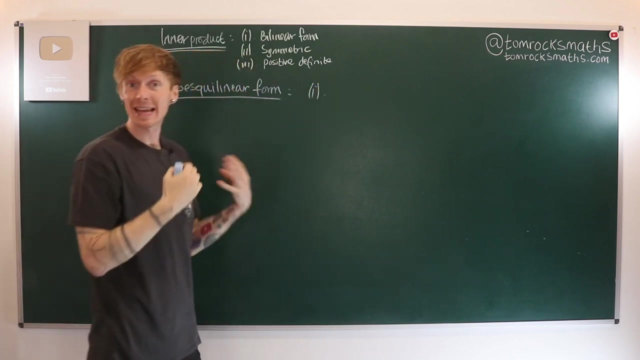 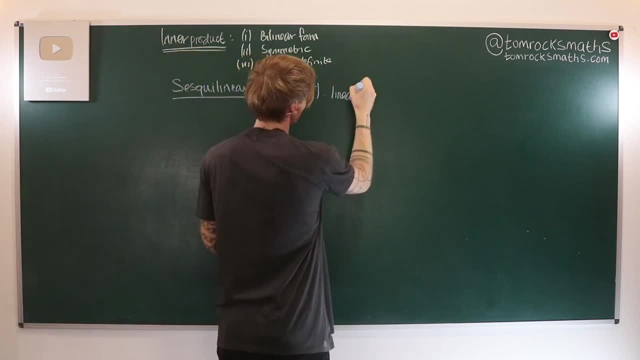 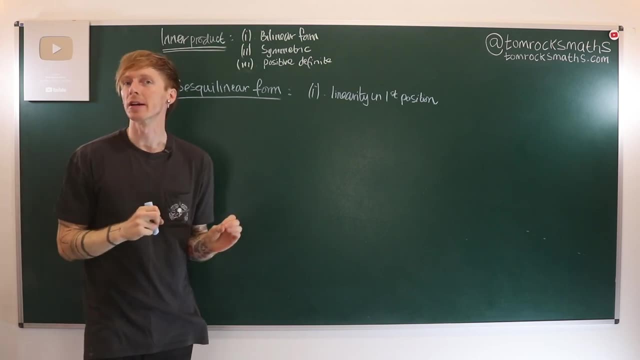 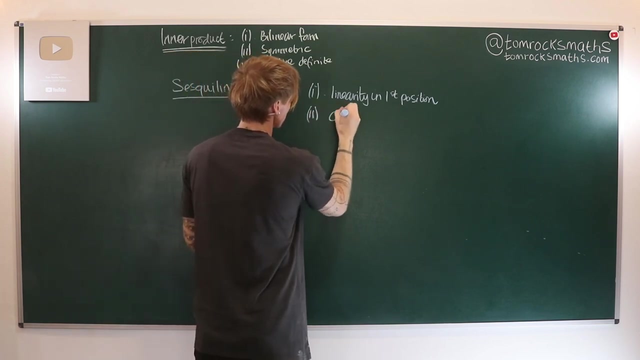 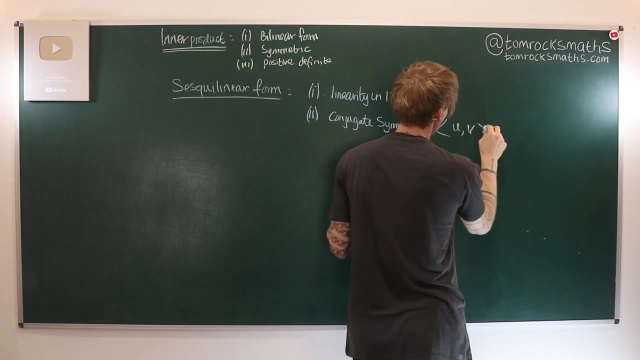 position. So linearity in the first position, but now our second property is no longer linearity in the second position, because instead we have something called conjugate symmetry. So this means that if I have two inner products, u and v- and I change their order, then that is the. 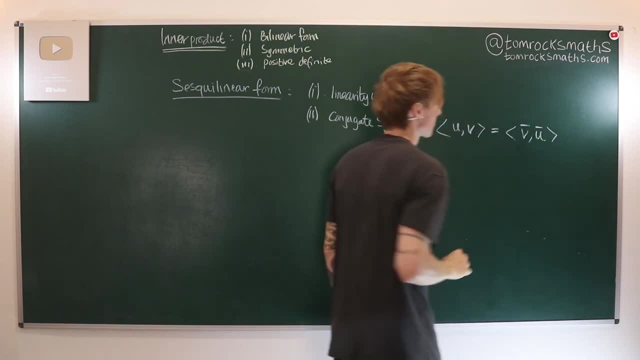 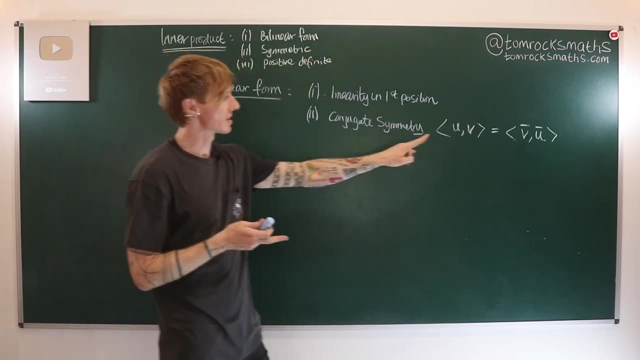 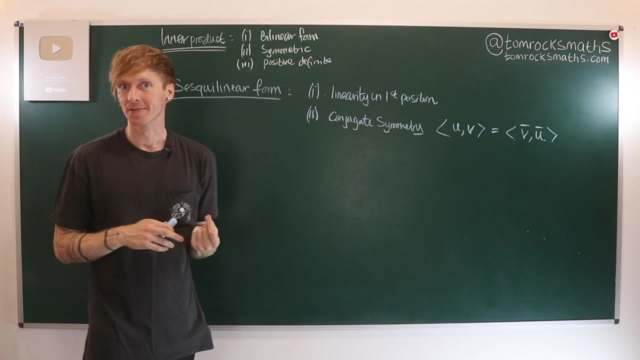 same as v bar u bar. So rather than complete symmetry, where they are equal when you swap them now, if we change the order we have to remember to take the conjugate of each of those elements when they swap position For the complex inner product space we again require positive, definite. 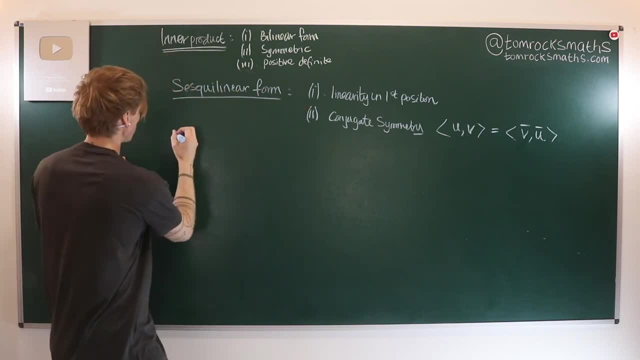 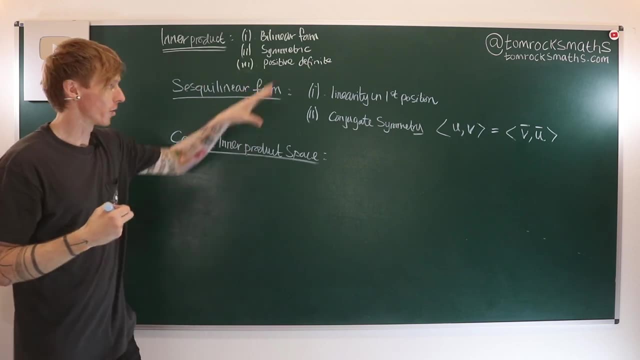 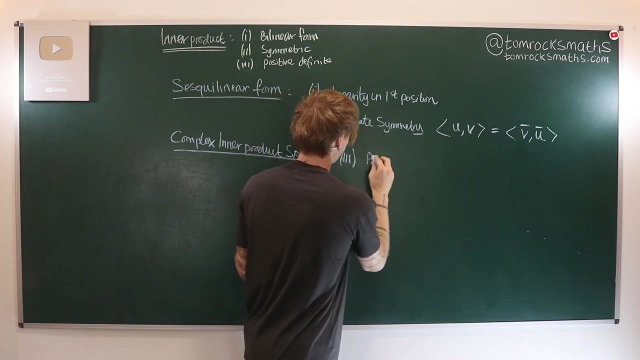 so these two give you your sesquilinear form. and then if we also want the complex inner product space, then that requires a sesquilinear form. so one and two, but you also need the third property, which is again positive definite. So the only real difference. 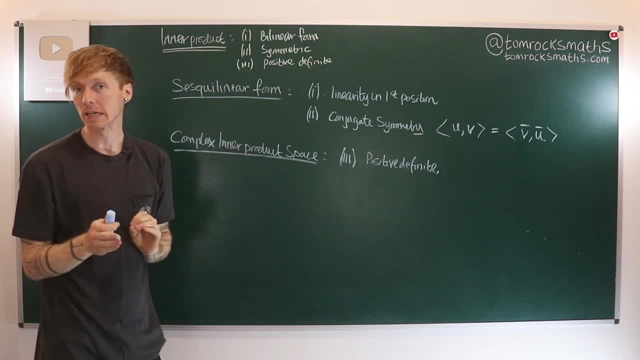 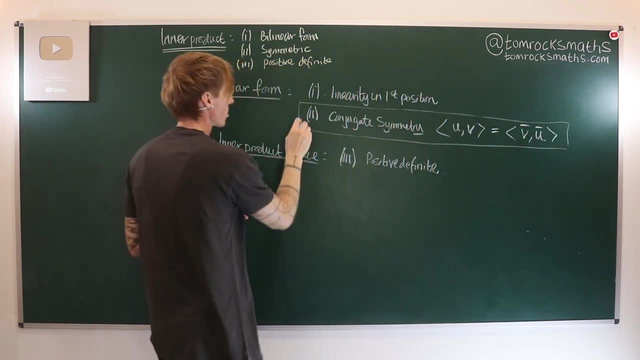 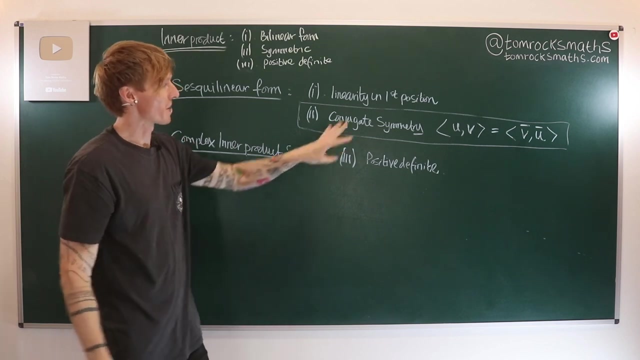 between the complex inner product space and the real inner product space is actually this conjugate symmetry. So now we can no longer freely swap the order of the elements within our inner product. We have to take the conjugate if doing that when we're working over the complex numbers. 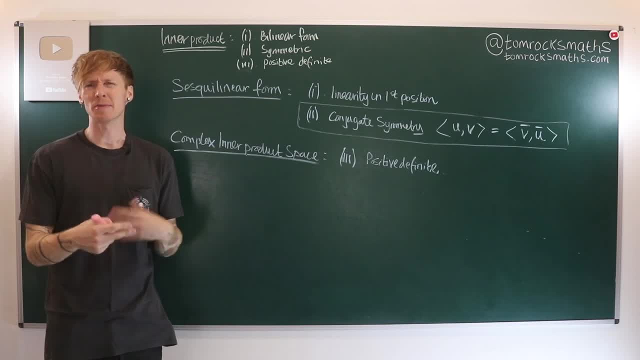 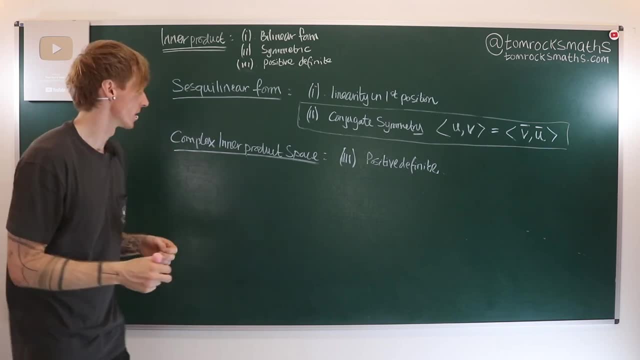 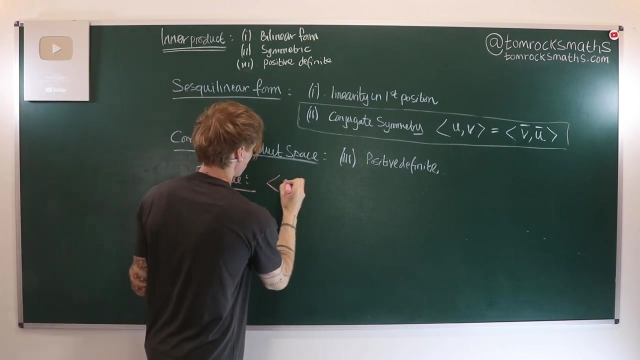 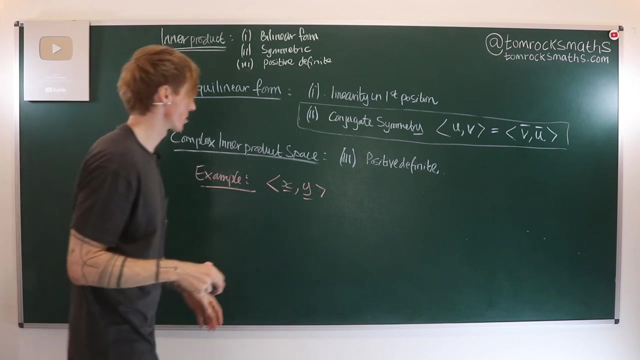 As before, the simplest example follows from something very similar to the dot product, just slightly modified: the complex number setting. So example: If we have two vectors, let's call them x and y, then we define the sesquilinear form or the complex inner product to be equal to. 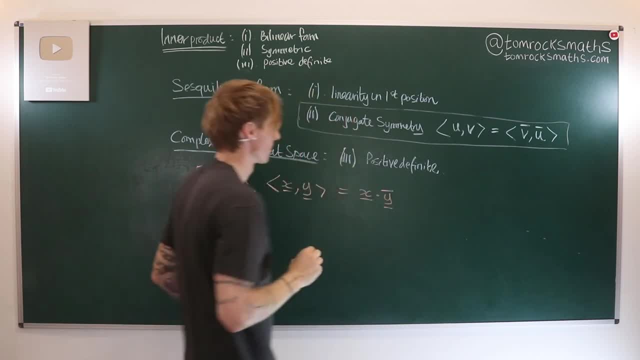 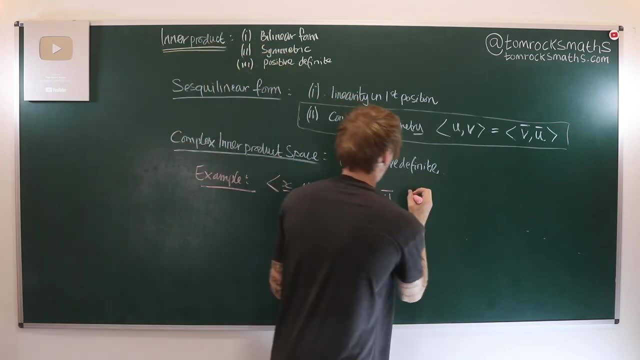 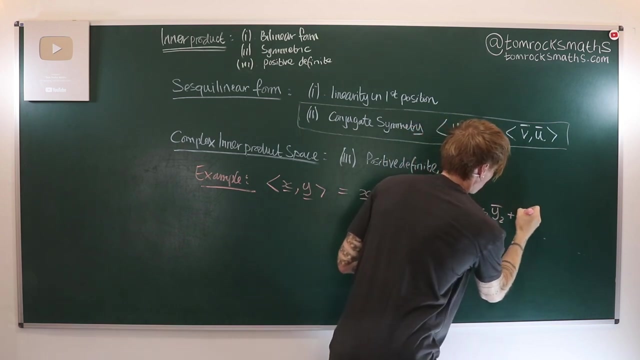 x dotted with y bar. So we take the dot product exactly in the same way but we have to conjugate that second entry. So if we expand this out, this would be x1 times y1 bar plus x2 times y2 bar plus dot, dot dot plus xn times yn bar. So very similar to the dot product. 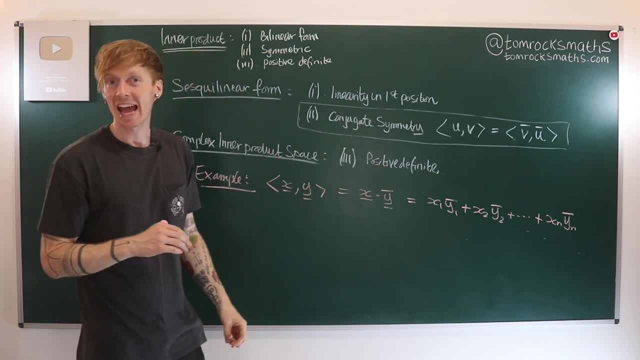 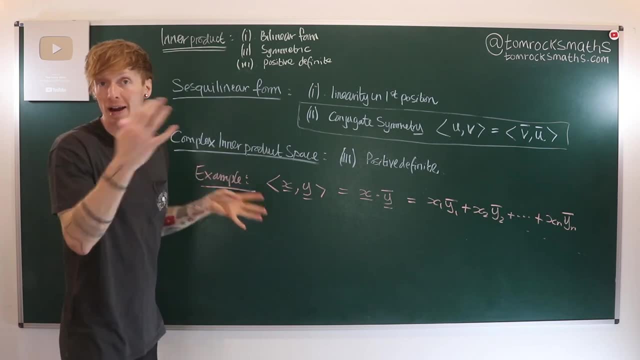 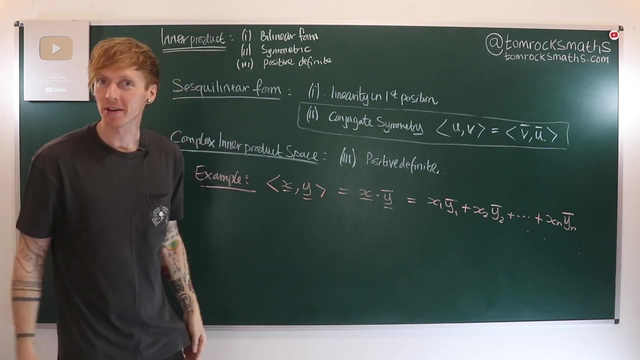 we just again put a conjugate on that second entry because now linearity will follow, exactly as before. and again I recommend checking this. I'm not going to go through all of the details because it's almost identical to what we did for the real dot product, but I will look at number two because 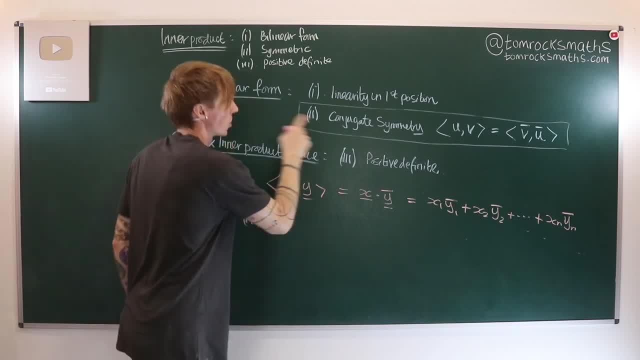 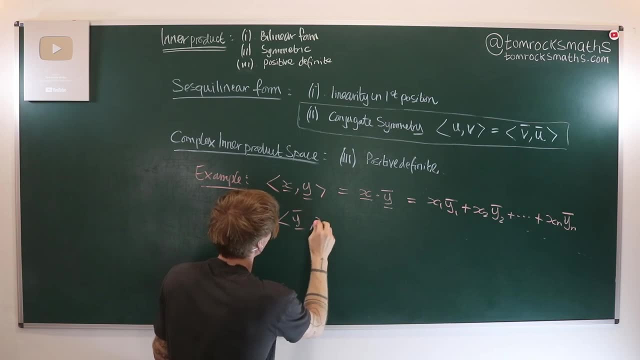 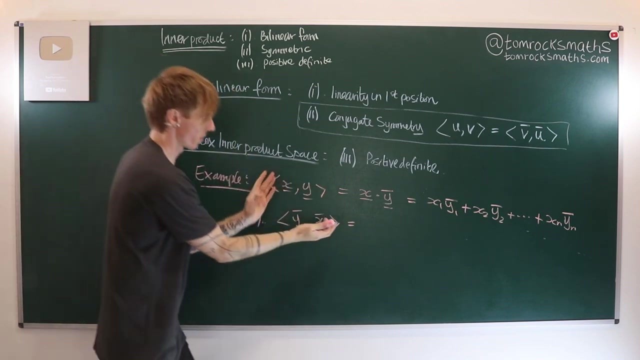 this one is the interesting one, the new one, conjugate symmetry. So if I now compute, well, what happens if I swap the order? So now I have y bar and x bar. So according to my definition of the complex in a product, I take the first entry, which is just y bar and x bar. I take the first entry. 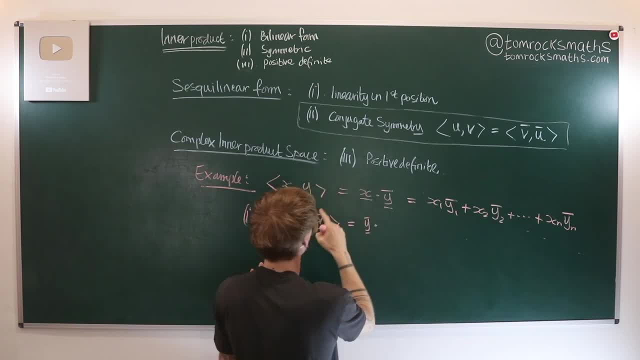 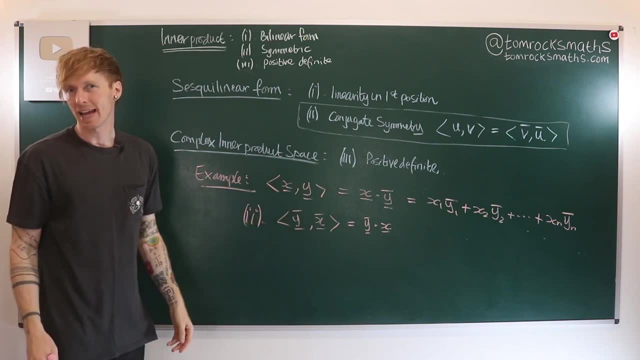 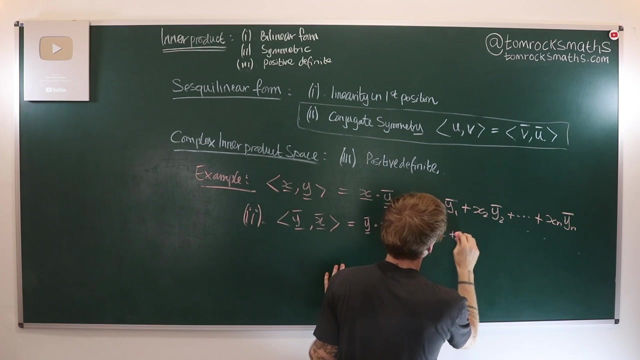 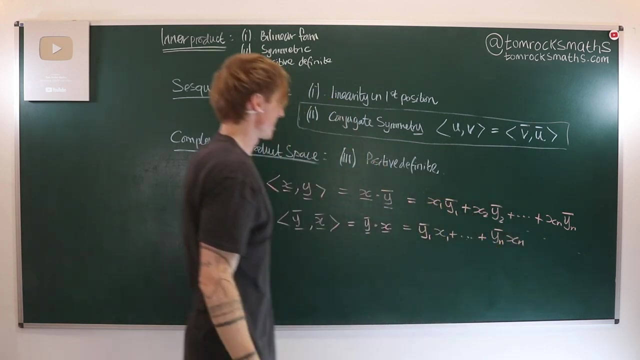 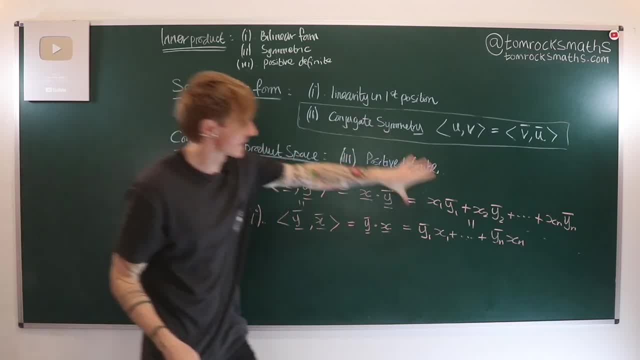 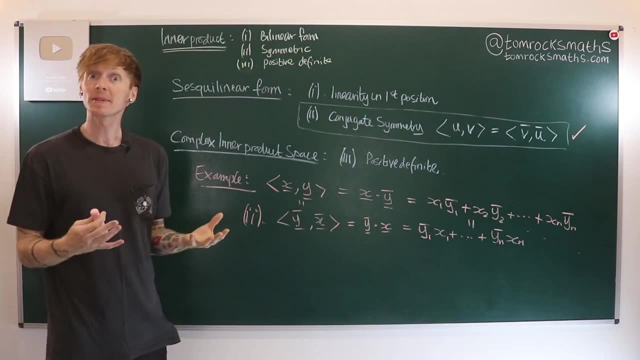 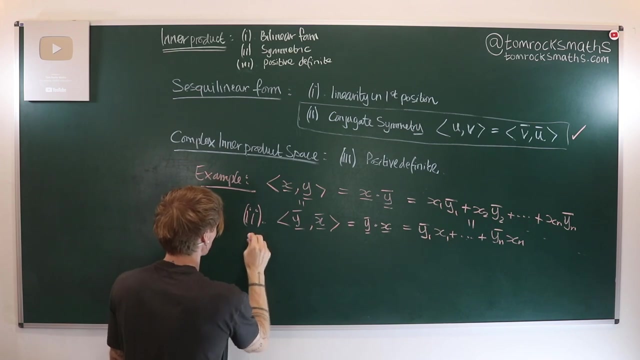 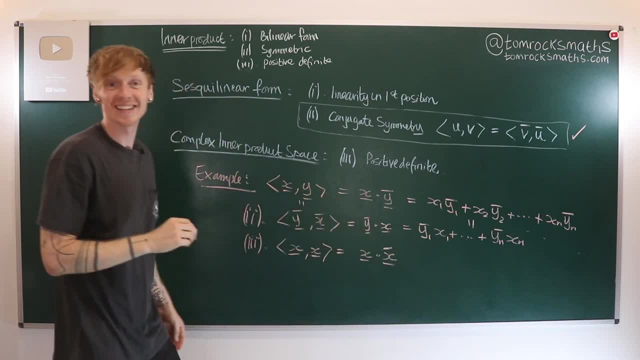 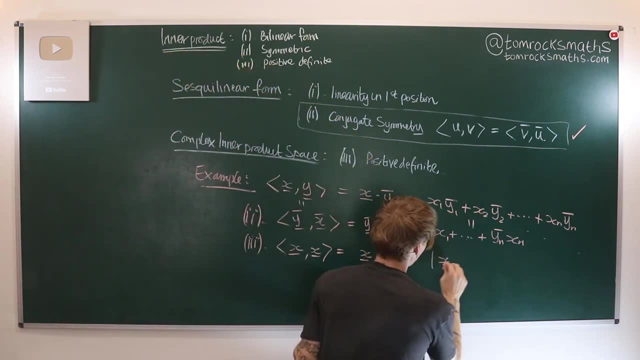 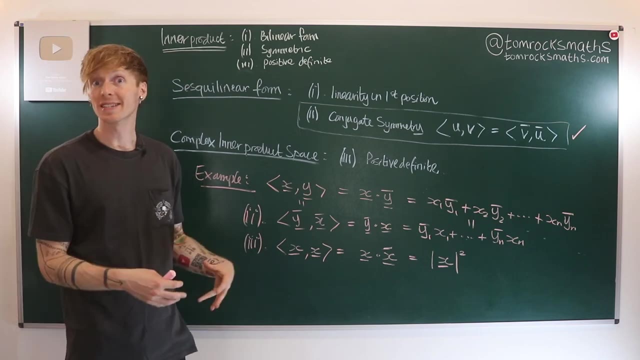 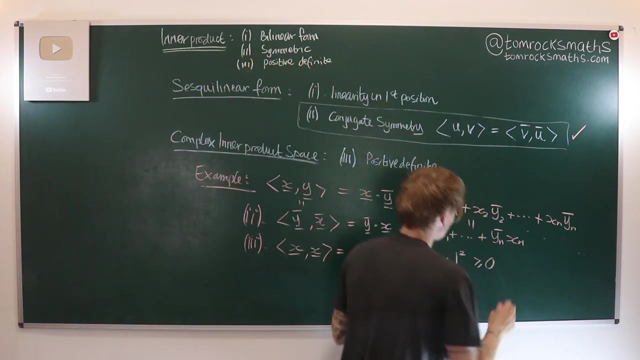